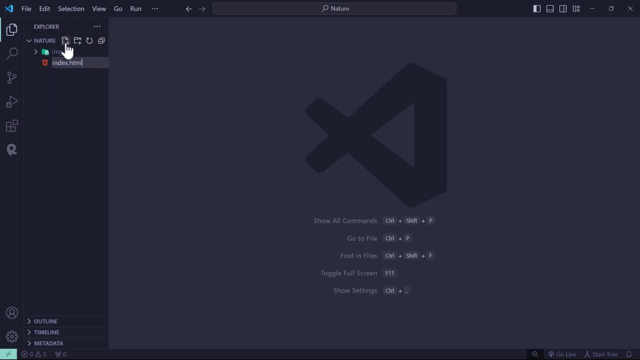 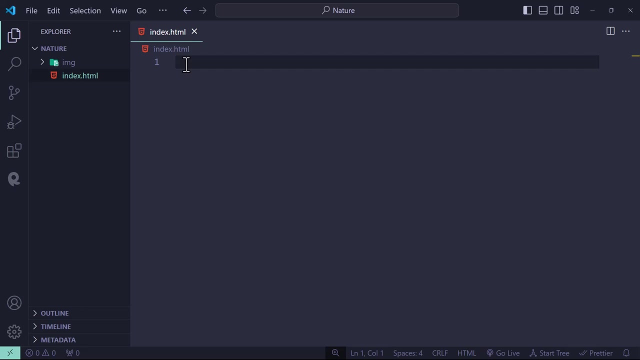 So I am going to select that And I will create indexhtml. Let me zoom in a little bit Great. And If you press shift 1 and And enter, This will create the default HTML boilerplate code for you, As you can see. 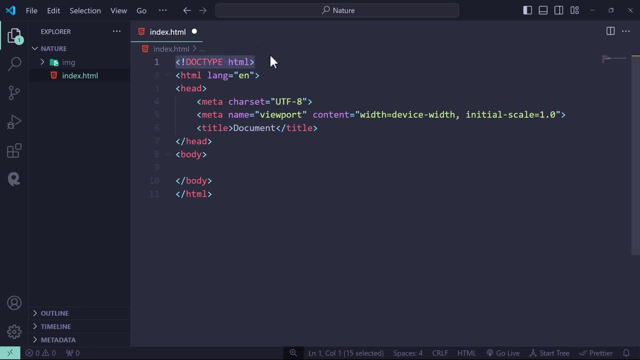 Doc type: HTML. This is the browser, that this is an HTML5 document And, as you can see, we have the HTML open and closing tag And head open and closing tag And the body tag And our title should be nature And inside body tag. 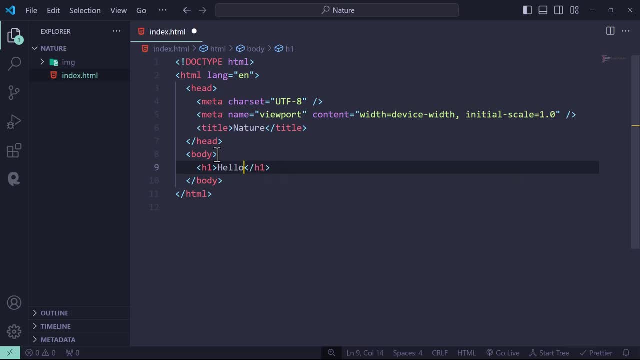 For now, let's create a h1. With hello world. Now let's create our CSS file And let's link up this CSS file inside our head tag. So just below the title tag, Link and press enter. Give the path to our CSS file. 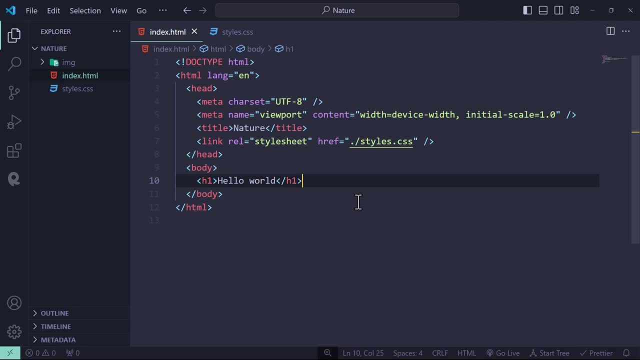 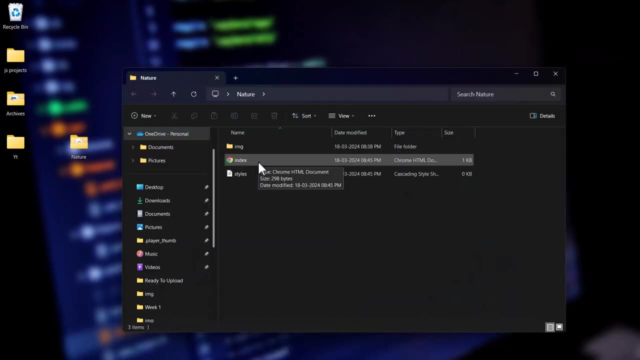 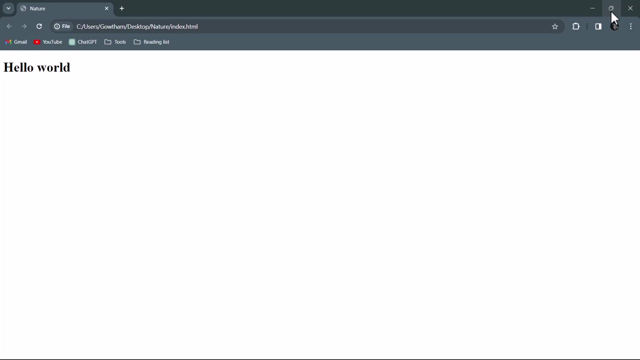 Now let's open our website inside browser. So to do that, You can simply go to your project folder, Double click on this indexhtml. This will open the project inside browser. So the problem with this is, As you can see, If I make any changes here. 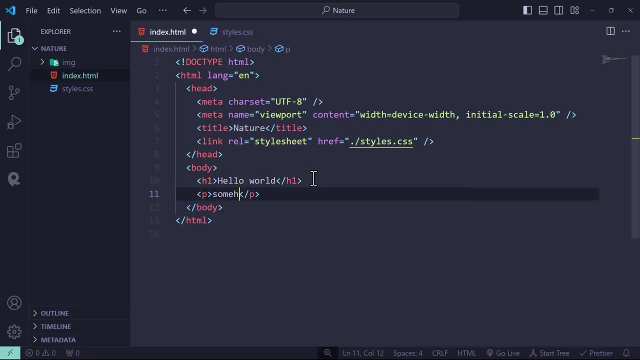 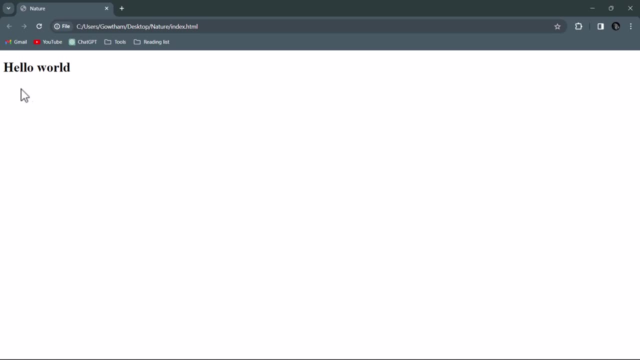 Let's say, if I add a paragraph Of something And if I come to our browser, You can see our paragraph tag is not visible here. So in order to reflect the changes we made, We have to refresh. So, without refreshing every time, 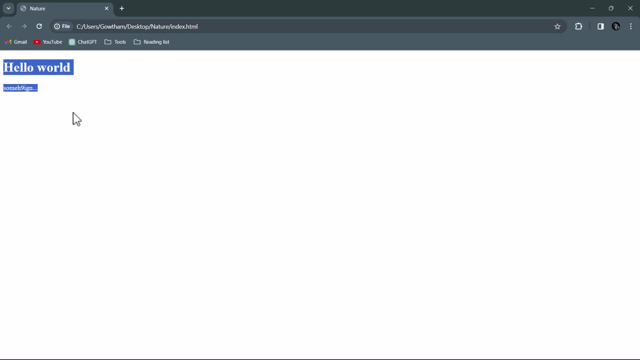 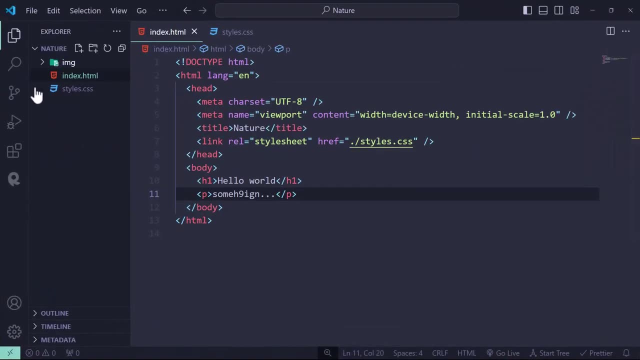 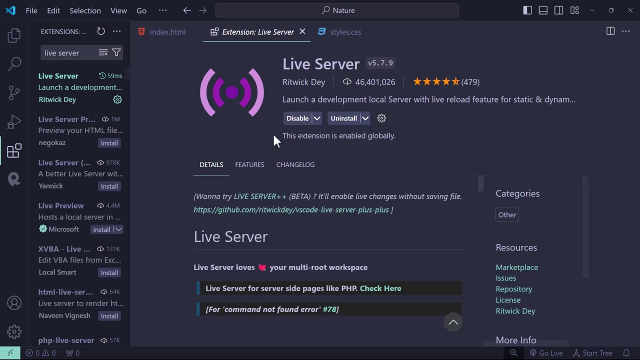 We want to auto update that inside our website. So to make that happen, Open vs code And come to this extensions tab right here And search for live server. You can find this extension. Simply install this. After installing it, Open your indexhtml. 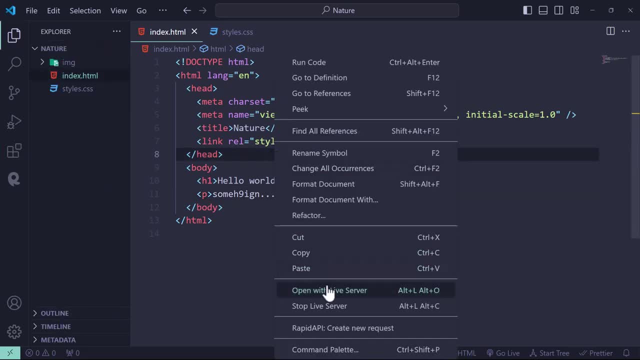 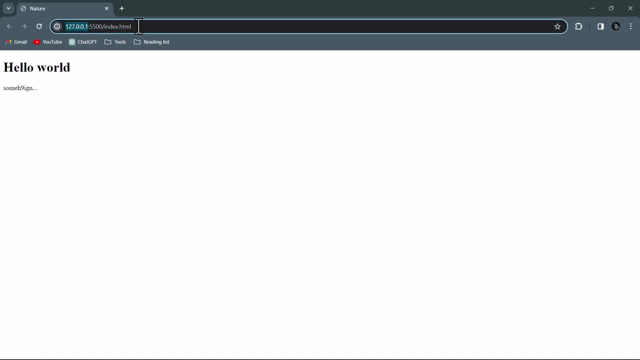 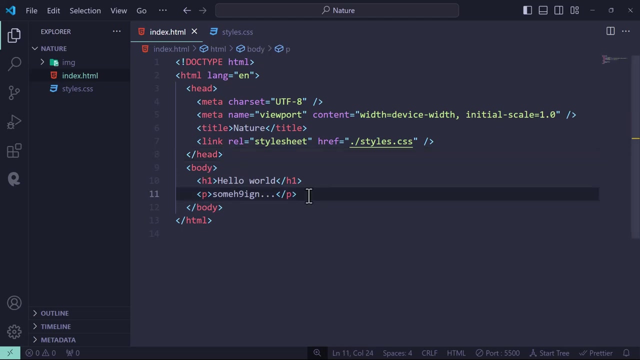 And right click And you can see: open with live server. Click on that. This will open our website inside browser. As you can see, This was opened inside localhost. Okay, Now, as you can see, If I made some changes, Let's remove this p tag. 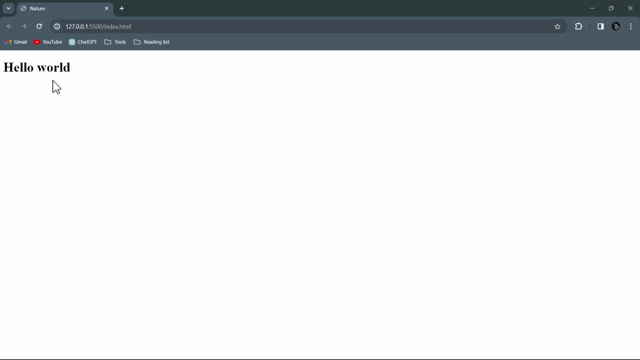 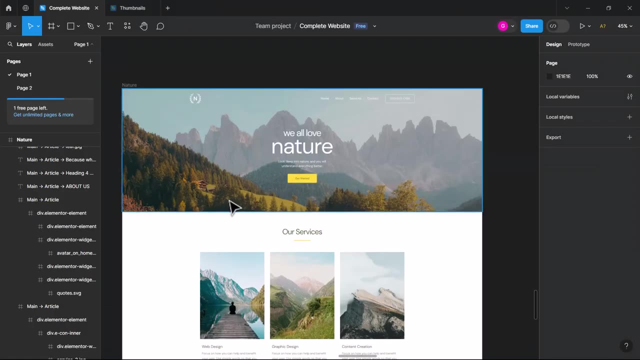 And save this. As you can see, It was immediately reflected here. Now let's start creating our website. We have this beautiful main section In which we have this nav And this background image And this header content, So Let's create a div for this entire header. 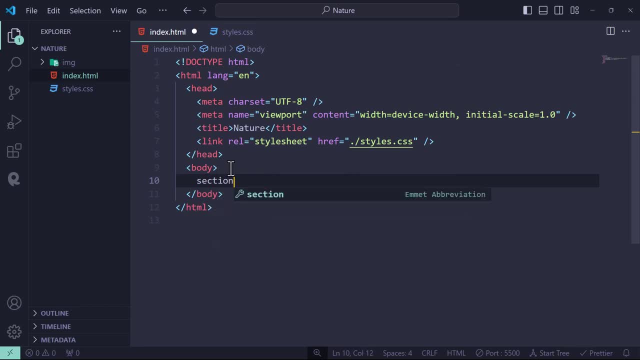 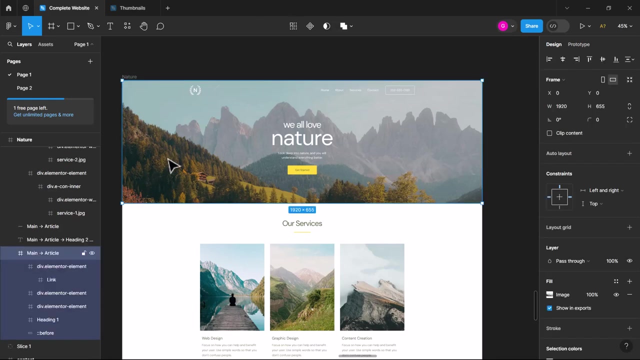 We will create a section with an id of main. This should be our main section And inside that We should have a container. This container is this entire thing. right here, See For the main section, We have the background image And this container should be this. 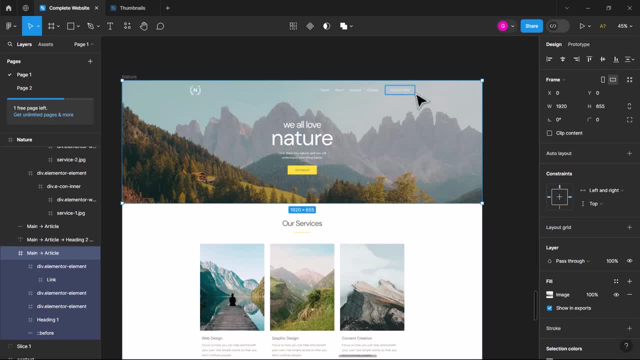 As you can see, Our button and this logo is ending up here and here Because of this, In which, Which is that, Which is the container that we are going to use Across our website. Our container has a maximum width of 1200 pixels. 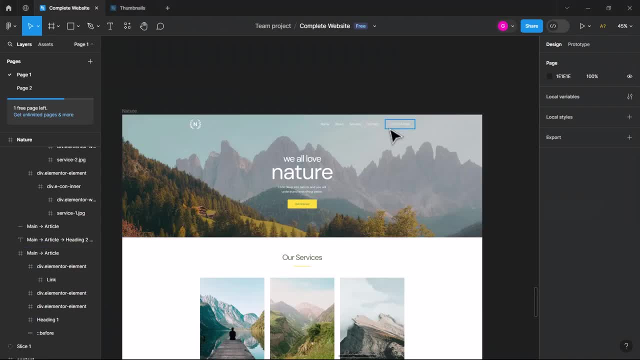 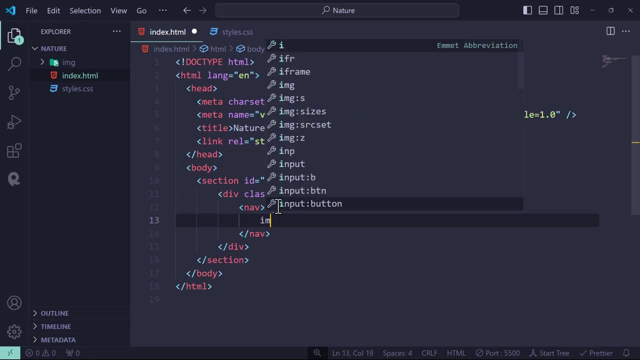 So inside that container We have this nav, So I will create a nav And inside that We have A image with a class name of logo In which We have inside images, Logopng, And after that we have our now list, which is an ul. this should be class name of now list in which we have 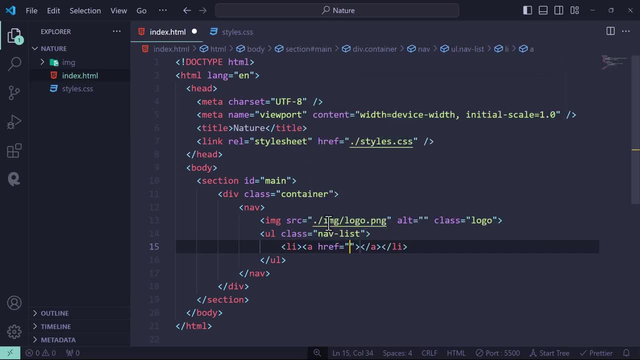 allies. each allies should have an anchor tag for now hash, and this is for home, and this is for network, and this is for services and this is for contact, and after that we have a button. see this button like here inside this on, i'll create a button with a class. 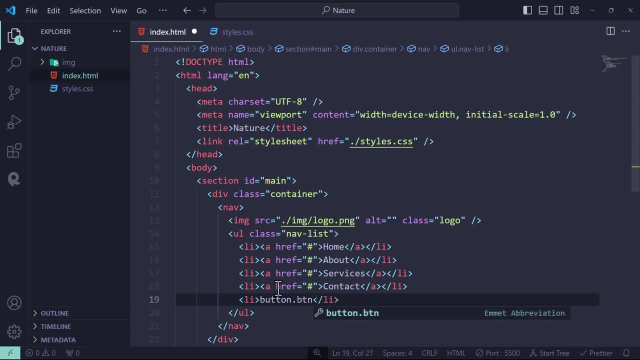 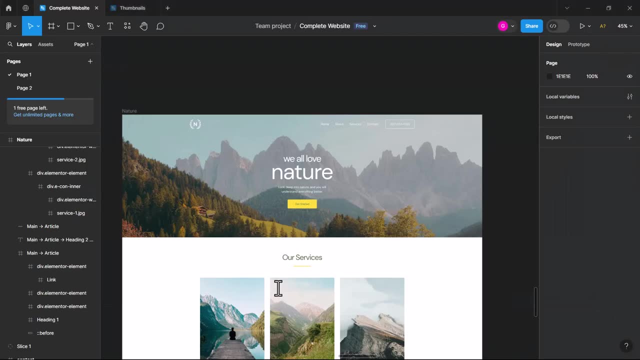 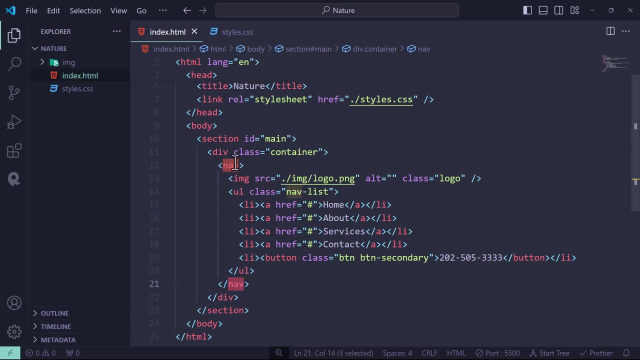 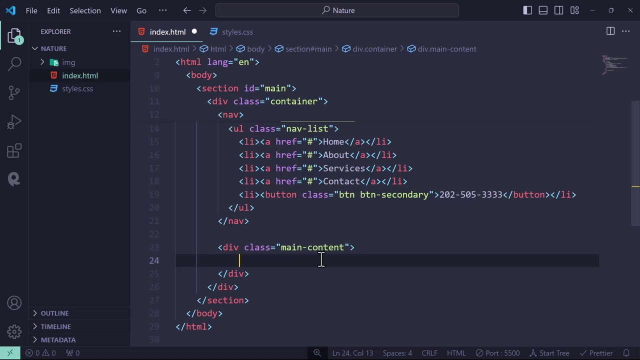 name of btn and another class name off btn, secondary, in which we have that phone number, something like that, and after the nav we have this main content. so i will create a div with a class name of main content. so in inside this main content with a class name of: 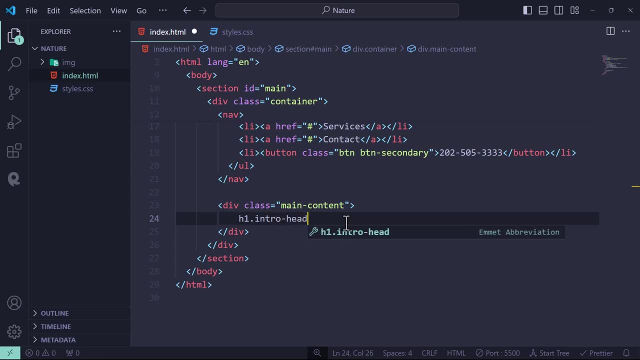 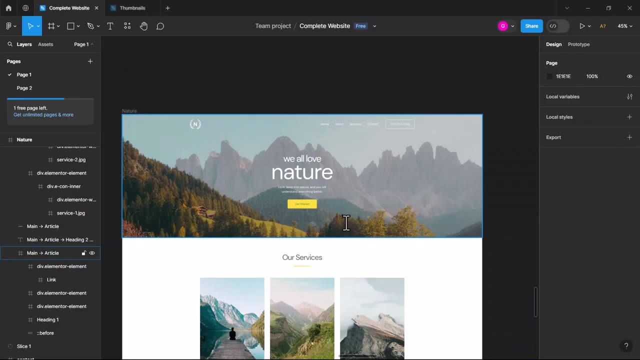 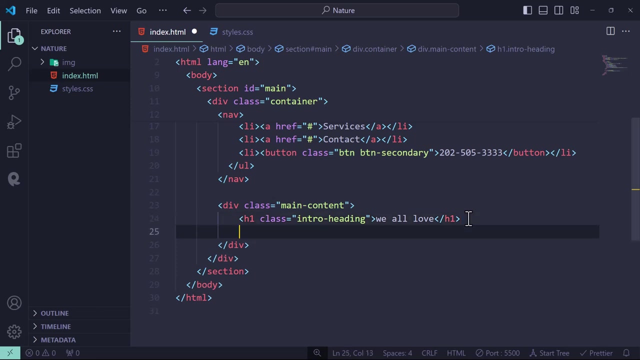 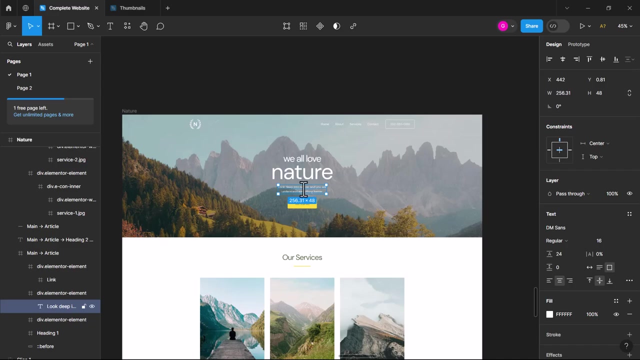 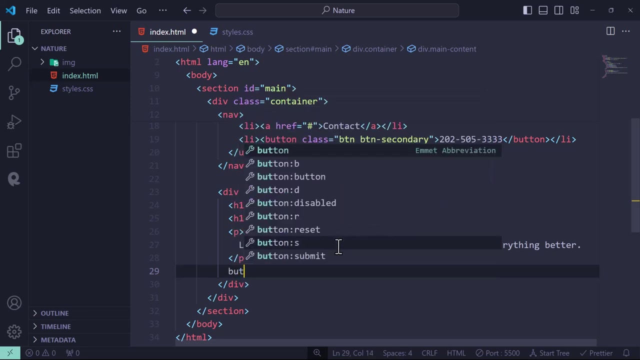 intro heading. this should be: we all love. this should be small letter and after that another h1 with main heading. this should be nature and after that we have a p tag with this text and after that we have a button with a class name of btn and btn primary. 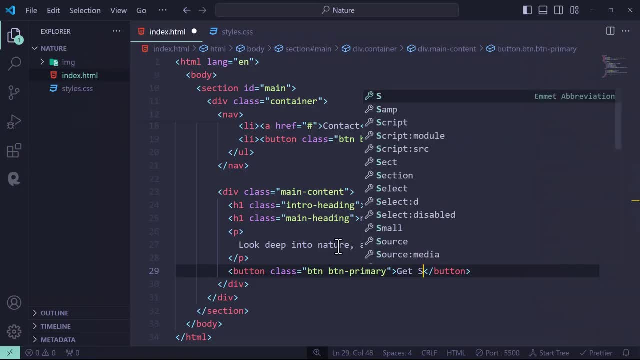 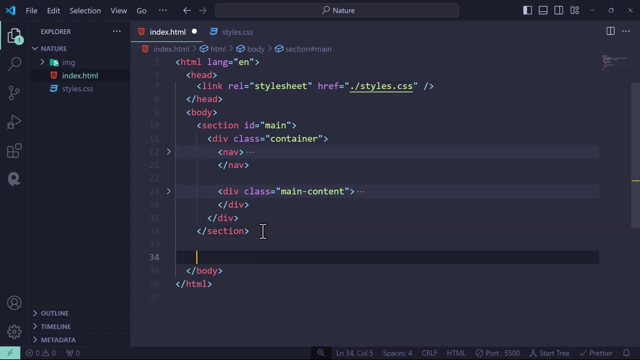 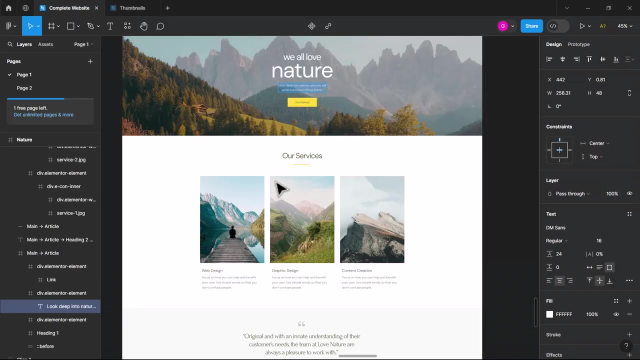 which we have get started, and after this section, which is this entire header section, we have a button which is this entire header section, which is this entire header section. we have our services section, so let's create a section with an id of services and inside this services section we have a container. 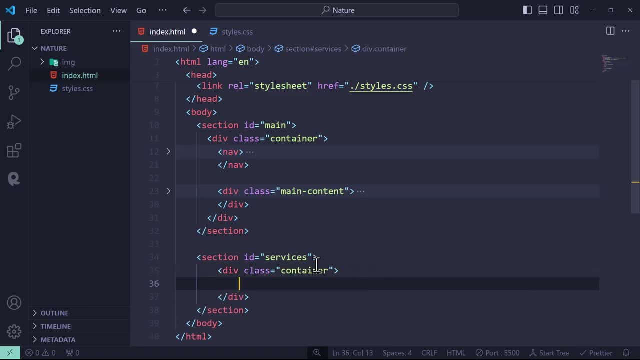 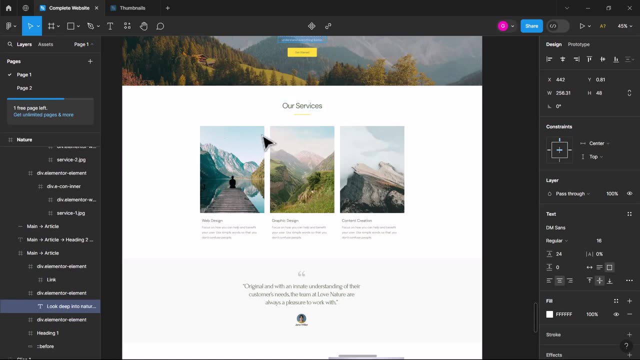 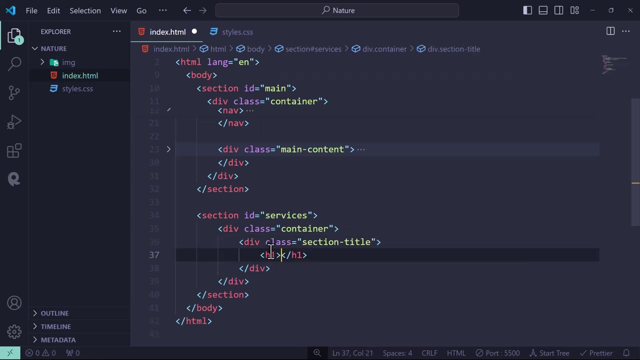 so i'll create a div with a class name of container and inside that container we have this h1 and this line right here. so for this entire thing, i'll create a div- section titles, and inside that we have a h1, this with the, the title for our section for services, and after that we have a div. 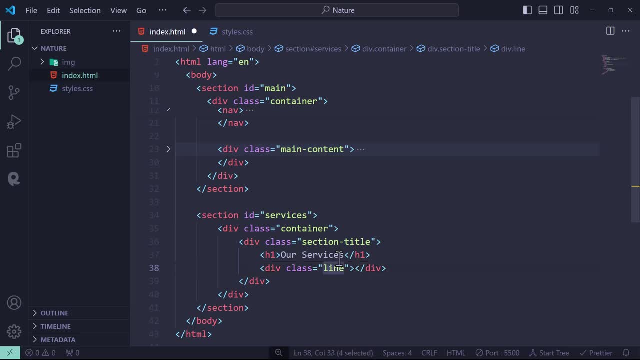 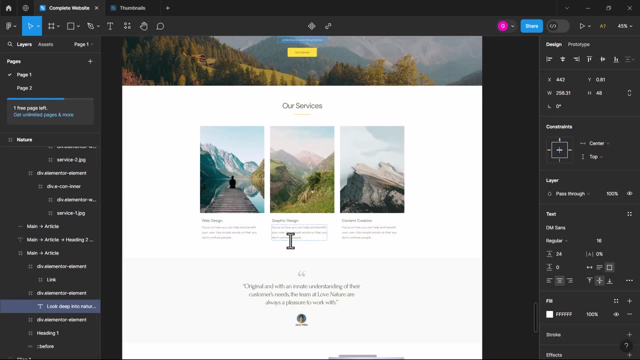 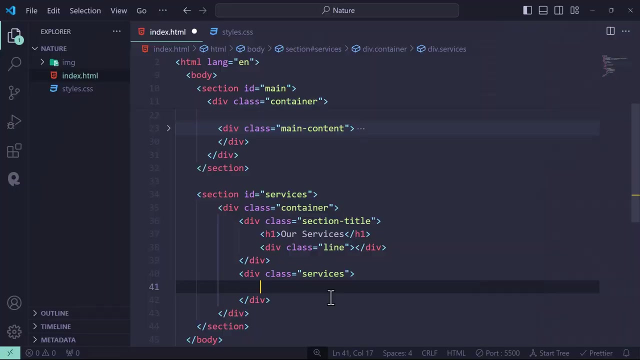 with a class name of line. we we gonna style this using our css. so after this section title, which is this entire thing, we have this services. so i'll create a div with a class name of services in which we have all of these three services. so let's create a service. 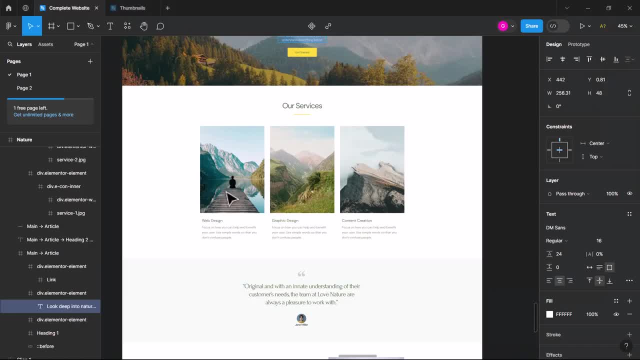 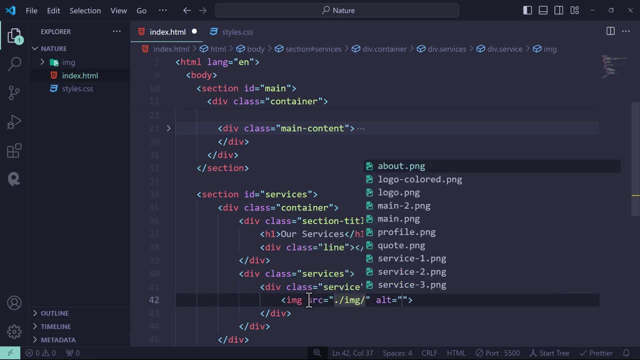 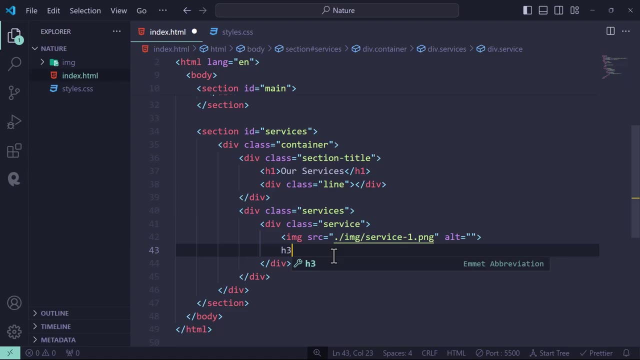 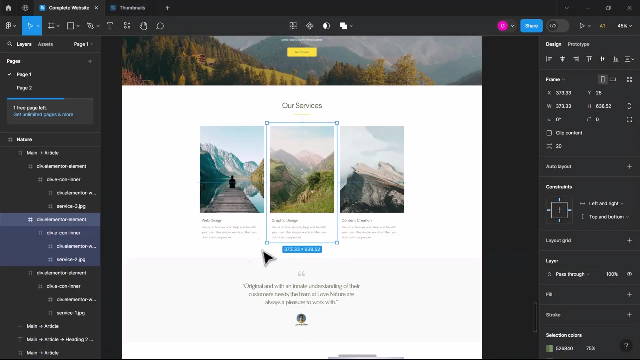 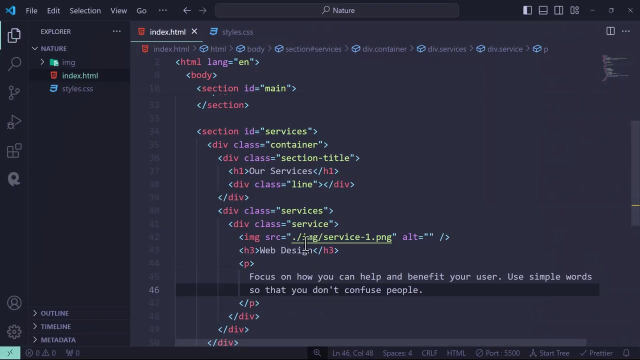 inside services. we have service in which we have image title and description, so i'm gonna add a image. this would be inside images service one, and after that we have h3 of web design, the p tag and a description of this text. let's duplicate our service, so simply copy this. 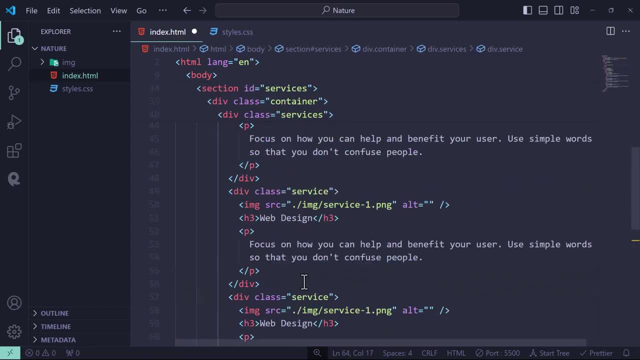 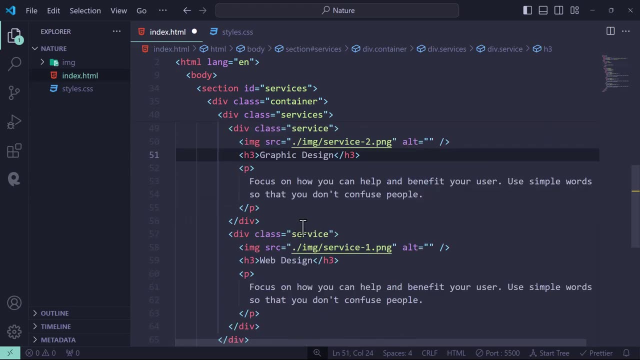 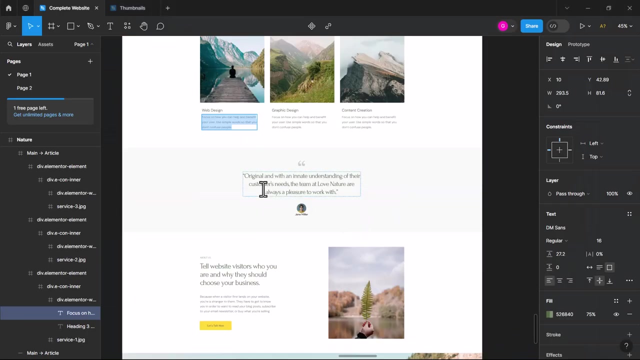 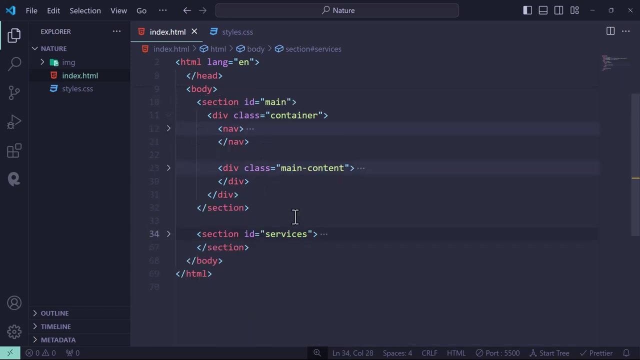 and paste it two more times. so this should be service two. this is for graphic design and this is for content creation and this should be service three. so after that we have this testimonial section. so after the services section, as you can see, this services section we have a section with a class name, with an id of testimonial. 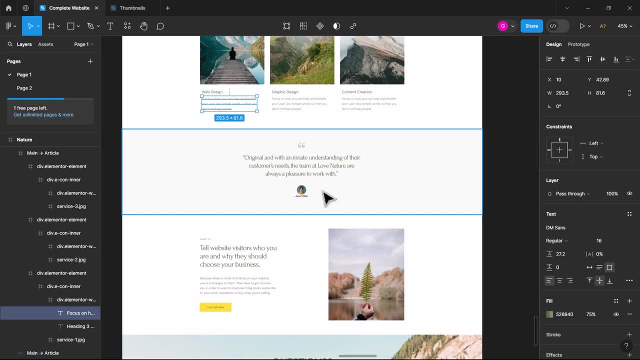 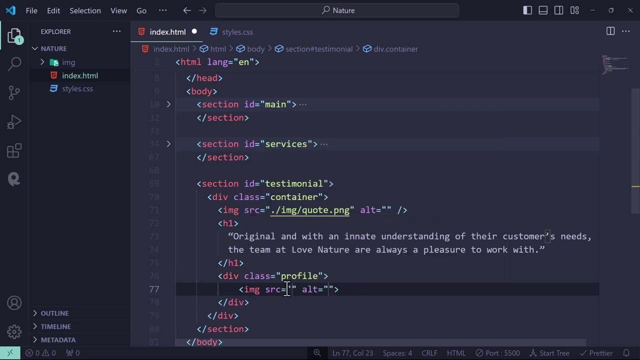 inside this testimonial we have this container. inside that container we have a image which is codepng, and after that we have a h1 with this text and after that we should have a div with the class name of profile in which we have the image. this should be inside images. 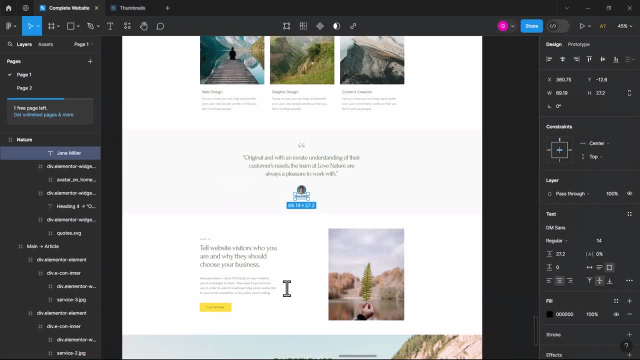 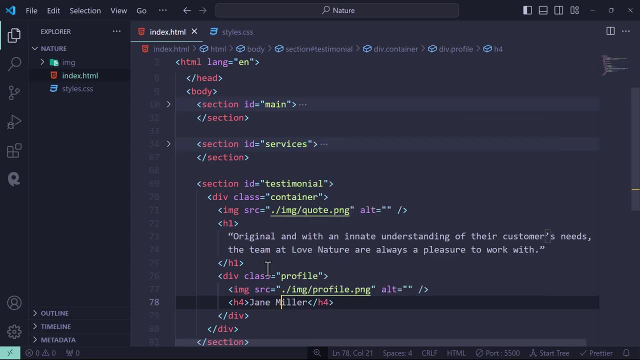 profile and ah4 with the text jane miller. after the testimonial section you can see on main section, services section, testimony and front end section. here we have a Superman font and what's on the front of the phone box inside the top. when we select雅 2 and then h4, we will see a again, x, Н. from the left we should see female�문 and female어를. we should see in imagesradius in it and ah4 with text Jane Miller. after the coronavirus你 видimo society. after the testimonial section you can see on main sections are first 2dx, sevFire Talk Oh Cameras, Levinfj RTKnik six haryl tipicom. 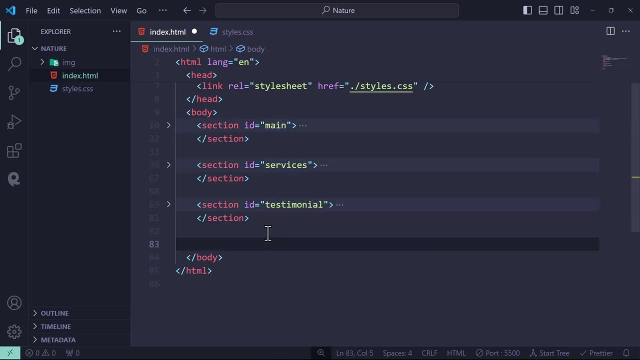 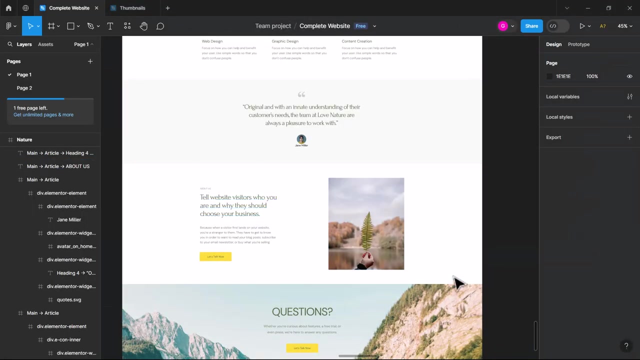 h4. you can see on main section, services section, testimonial and free news about HTML and katastrof, advertisement etc. section, and after that we have this about us section. so i'll create a section with an id of about us and inside that we have this container. 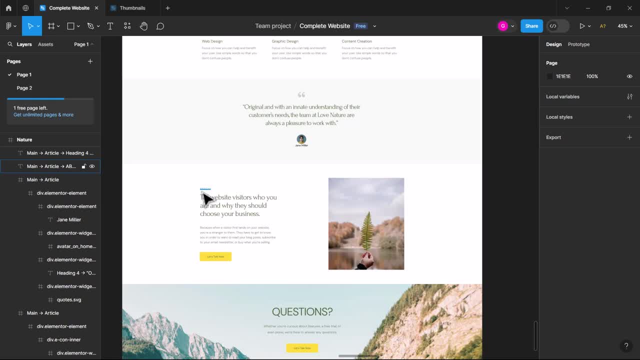 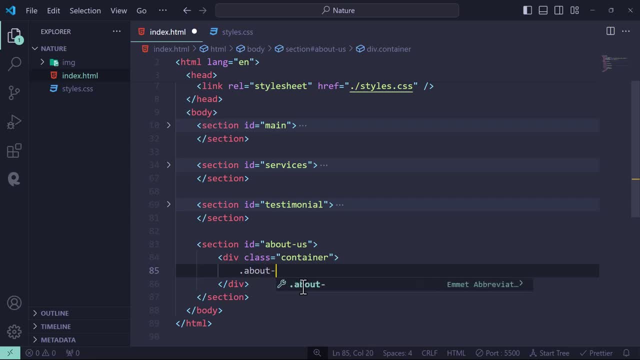 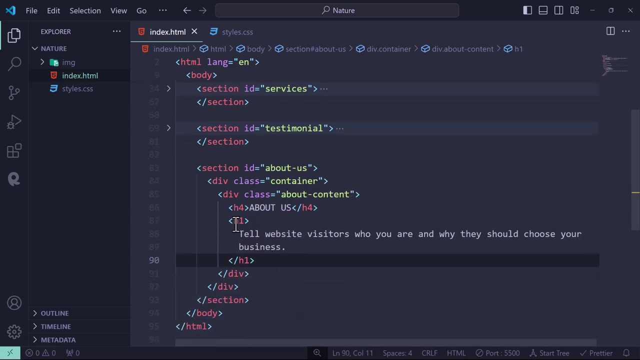 and inside that container we have this about content and about image. so i'll create a div with the class name of about content, which is this entire thing. so we have a h4 that should be about us, and after that h1 with this text, and after that we have a p tag. 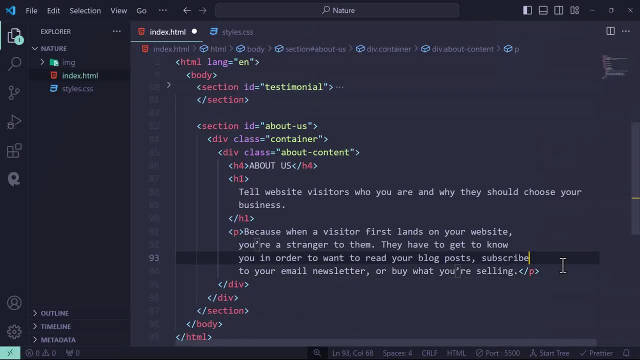 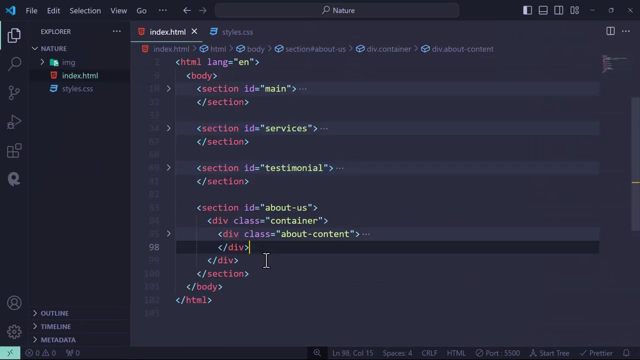 with the text right here and after that p tag we have a button with the class name of btn and btn primary in which we have- let's start now- and after this, about content. so i'll create a div with the class name of about image in which we have a image which should be inside img about dot png. so after the about section, 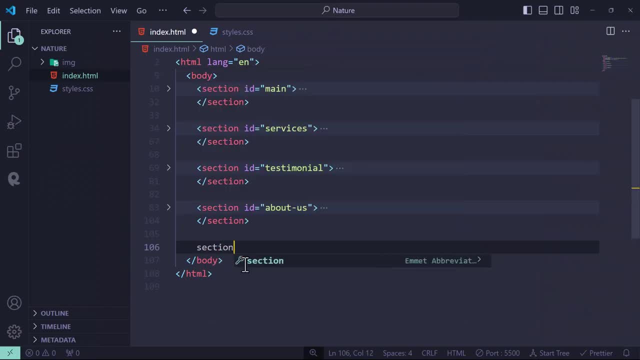 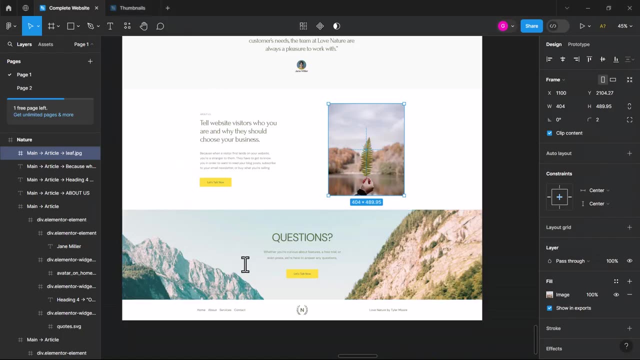 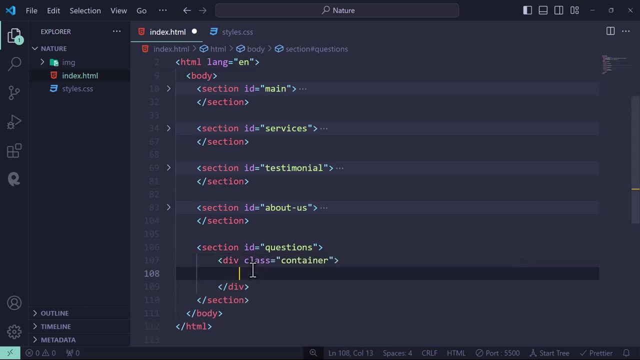 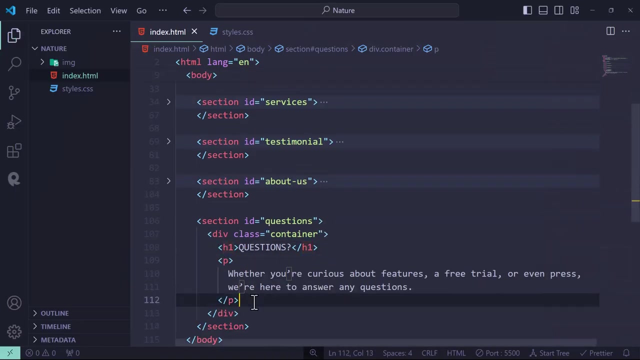 we have these questions, so i'll create a section with the class name of questions, so in which we have a container, said that we have a h1 with the text questions and after that we have a p tag with this text and after that we have a button with the classname of btn and btn primary. 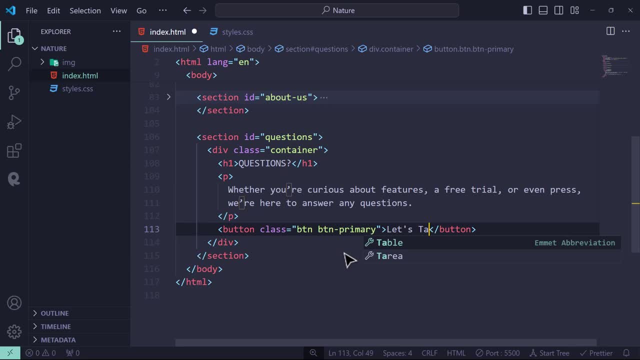 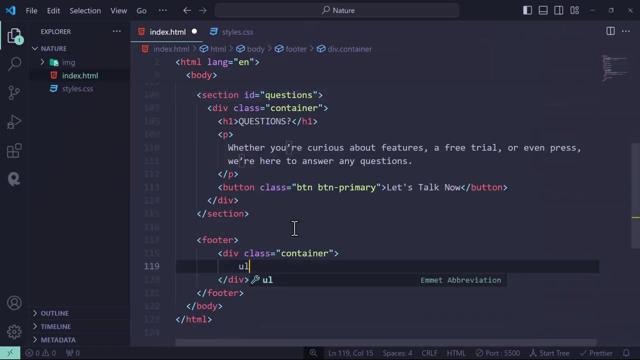 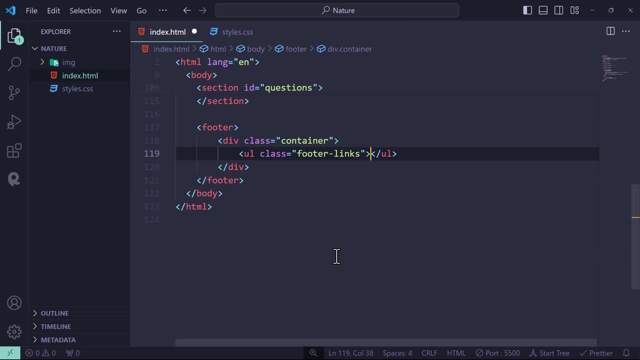 this should be. let's start now and after this question section. we have this footer, so I will create footer inside that. as you can see, we have a container. inside that container we have footer links. I will create a ul with a class name of footer links and in which we have an ally with an anchor tag of home. this should be about this. 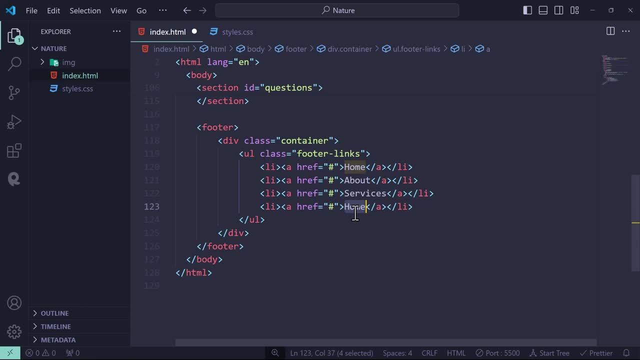 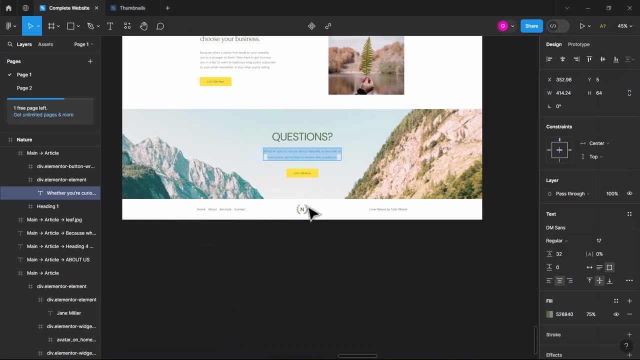 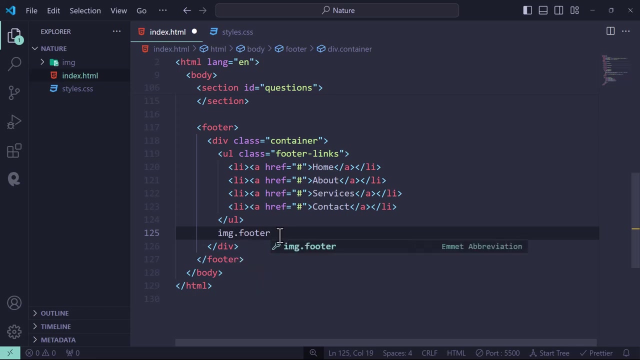 is for services and this is for contact. so after the ul, inside the footer content, after the ul, we have this logo. so I will create a image with the class name of footer logo and in which inside images, logo, colored dot png and after that we have this p tag. great now. 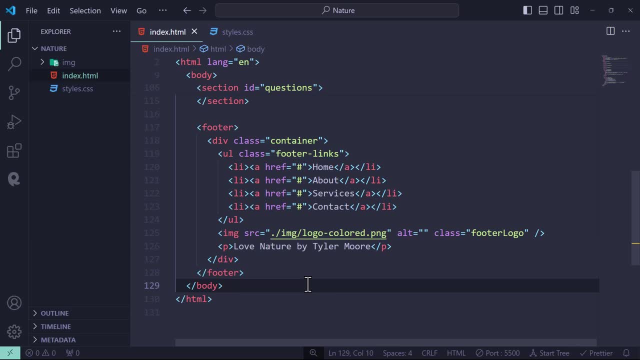 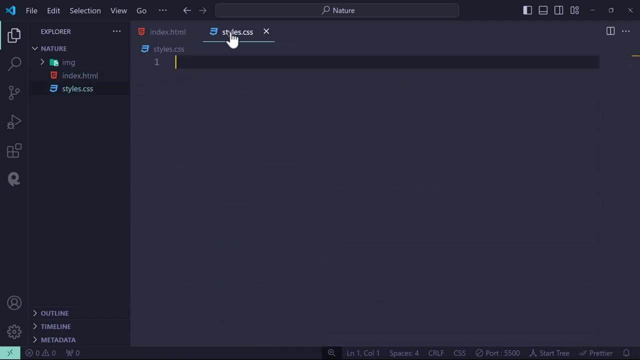 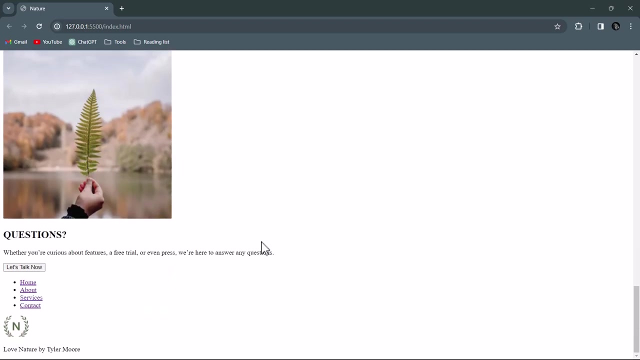 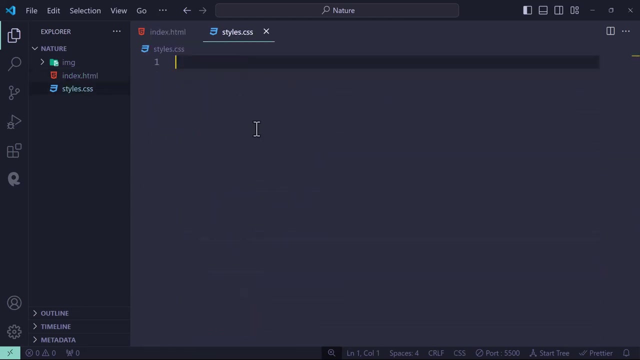 we designed our entire HTML layout. now let's style this inside our CSS. so to do that, let's make sure our CSS file is linked up. let's open this inside browser. so this is our website, without any css. now we are going to make it beautiful using our css. okay, let's open our css file. 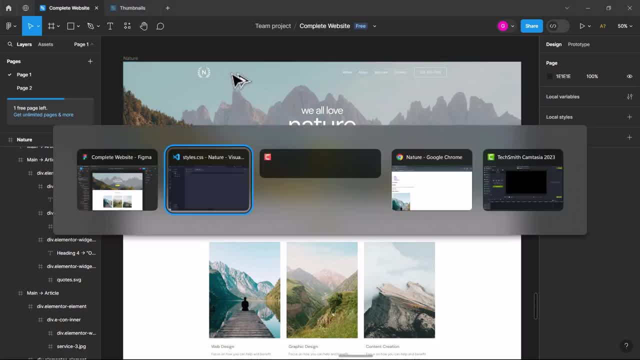 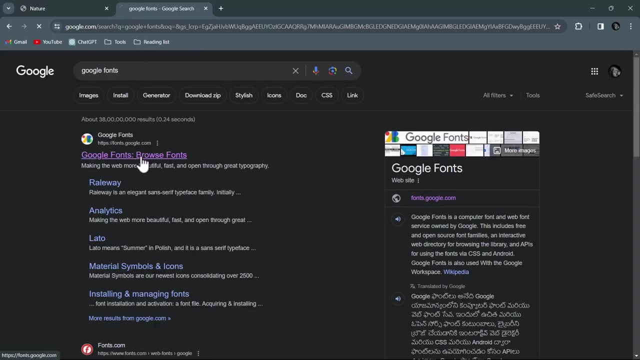 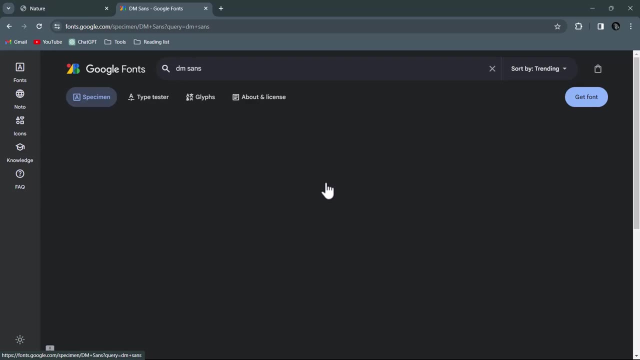 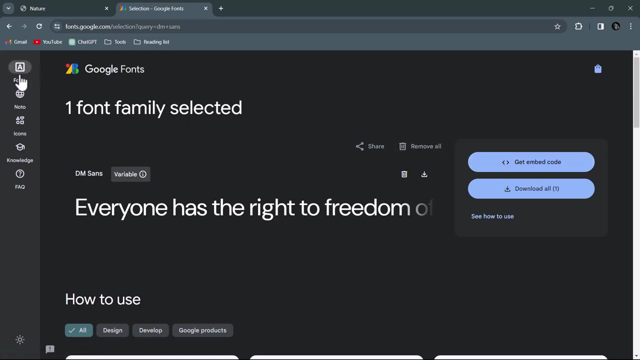 at here. we need two fonts from google fonts. so open your, open your browser and at here search google fonts and you can find this first link right here. open that and search for dm sans and select that, click on get font and again go to fonts and search for forum and click on it and 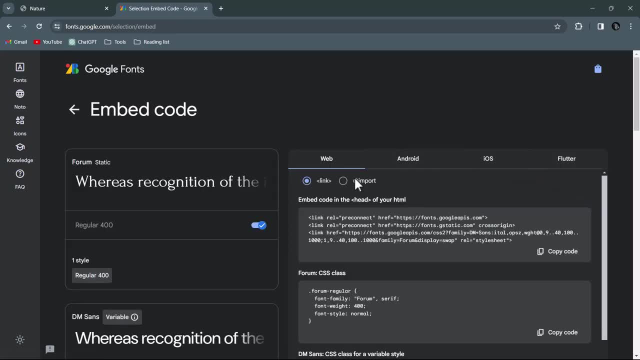 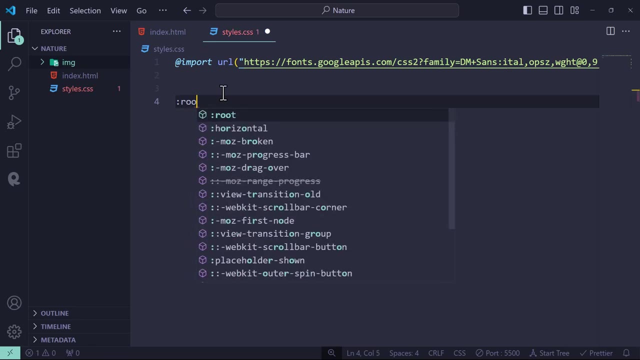 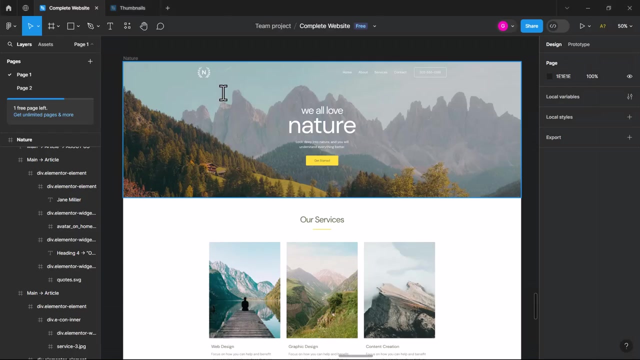 click on get font. you can see at here. on the import, you can see dm, sans and forum. so simply copy this and paste it here. now let's create a root, our root variables, in which we have color primary. for this we have this green color. i'll copy that. 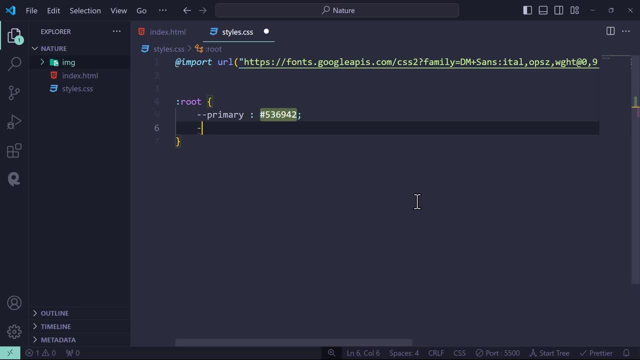 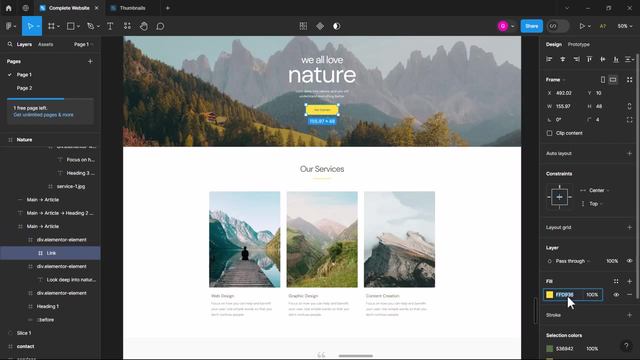 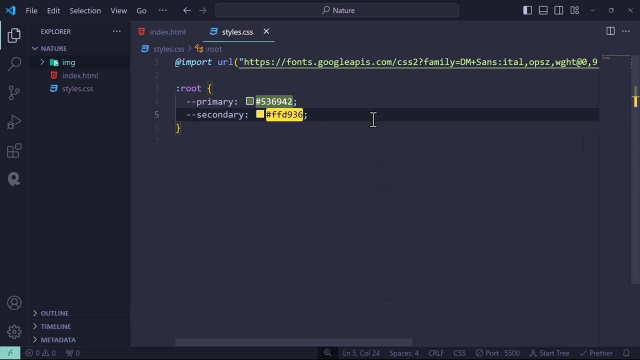 and paste it here, and after that we have a secondary color, which should be this color. these are the two main colors that we are going to use, and i'll create a color of white. this should be ef, ef, ef at here. as you can see, our every single html element has a default margin and paddings. 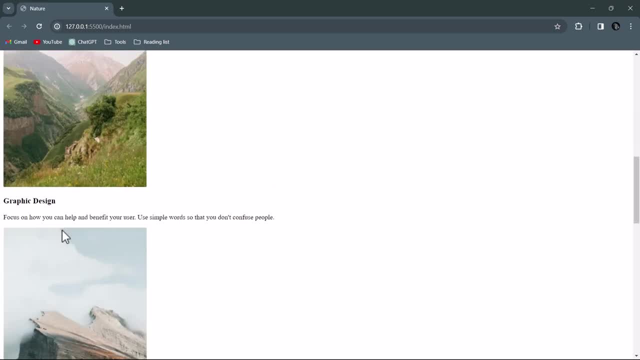 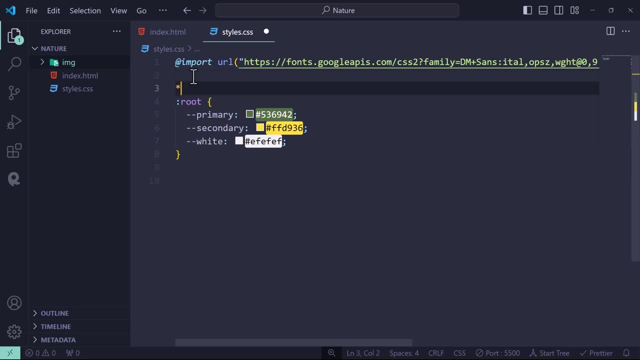 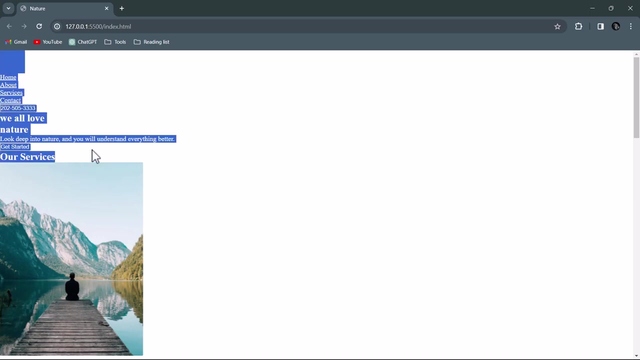 as you can see, there is some kind of space between each of these elements. so to remove that, the top right here for hashtags make margin zero, padding zero and box sizing border box. so this will remove all the default margin and paddings for each and every single element inside inside. 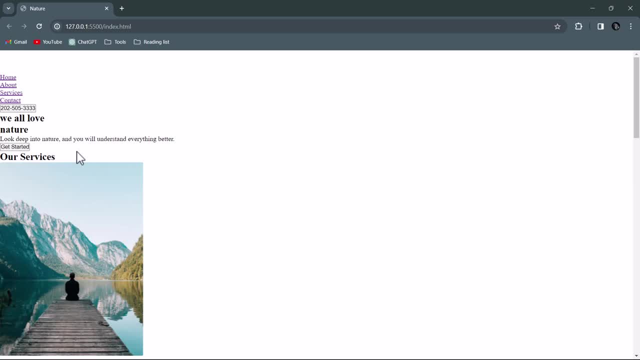 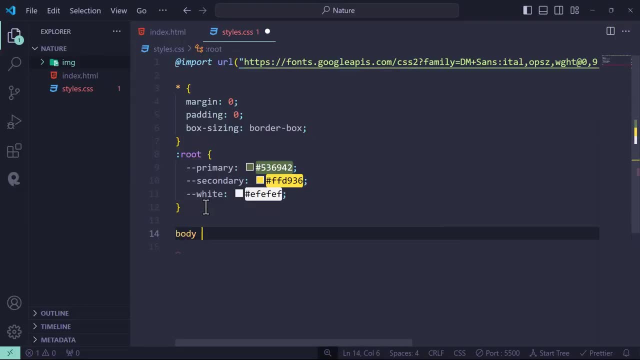 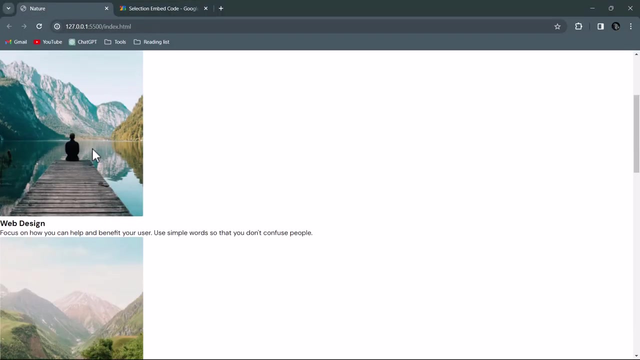 our html. so. so now we can give whatever margin and paddings that we needed for every specific element. so at here for the body. first, let's make font family. let's make font family here here: dm and sans, and, as a fallback, sans-serif. as you can see, we have this dm sans font. 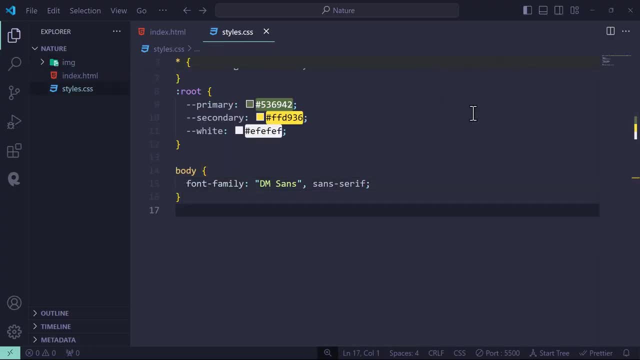 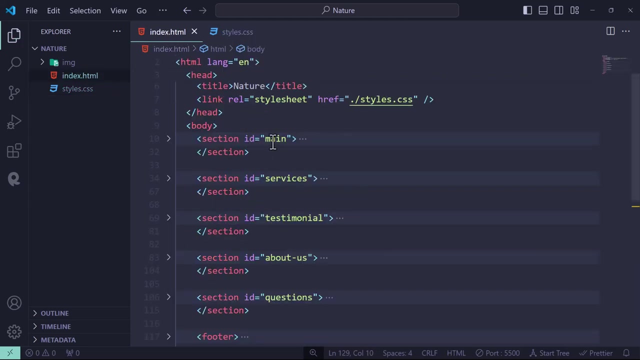 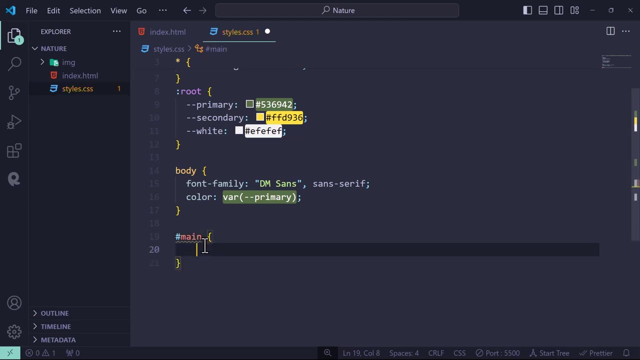 and for every text inside HTML. we should have a color of primary only specifically for our nav links, except that everything has this color by default. so after that, inside our nav, if you remember, for this section we have an id of main. so for the main section we have a background image. this would be. you can give background image by this property called. 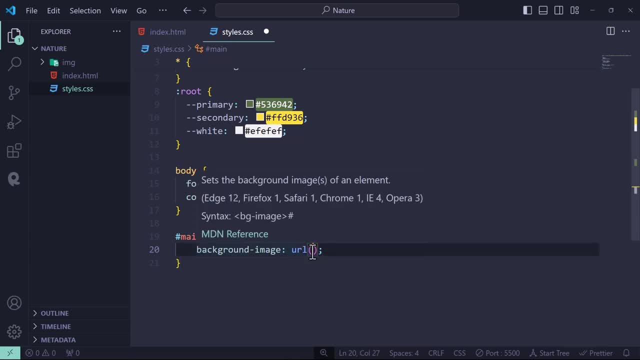 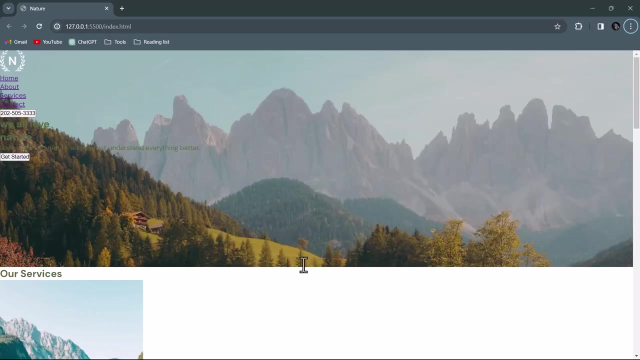 background image and url and inside this you have to give the path for the image. inside images, mainpng. and if you open the browser, as you can see, we have this background image here. so for this we should add a minimum height of 70 vh and background position, bottom center and background size cover. so now you can see we have this beautiful. 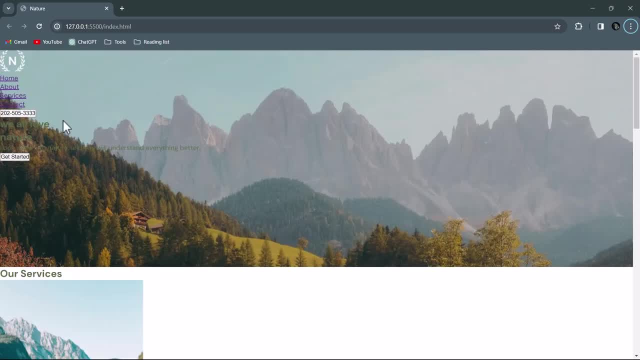 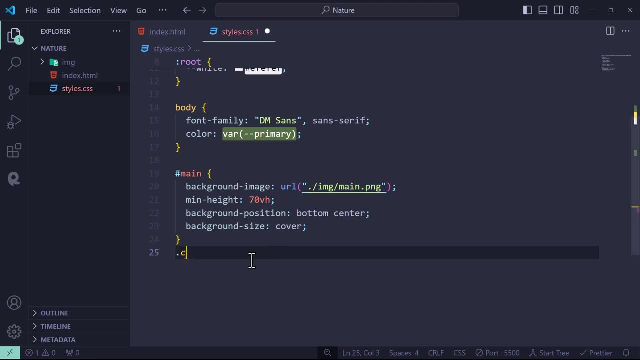 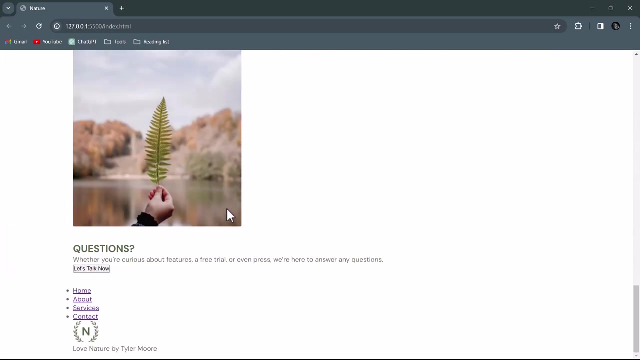 background image on top of this. we have this: our navigation and our entire navigation is inside container. so for the container, we'll add a max width of 1200 pixel and a padding of 16 pixel and margin auto. you can see this more: entire content to a maximum width of 1200 pixel. so inside 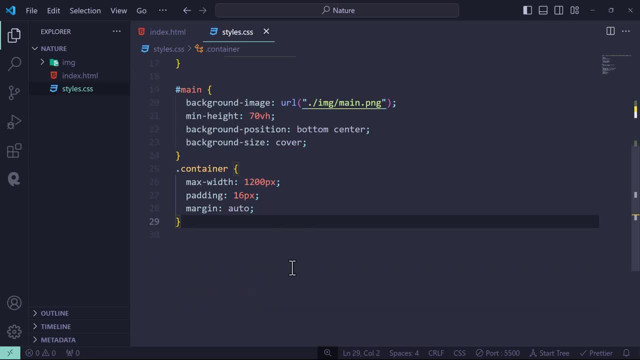 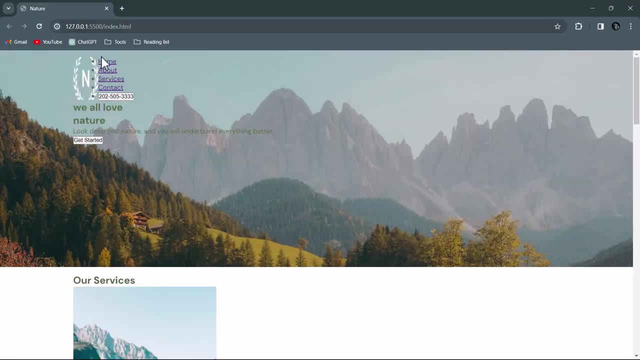 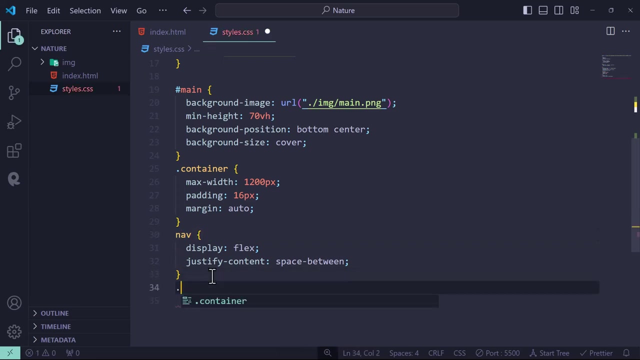 this now, which is this now right here, we should make display as flex so that it will line this logo and this now links side-by-side and if you make justify content space between, that will align the logo at here and the now links at here. so inside now we have now list for that. also, if you make display flex, 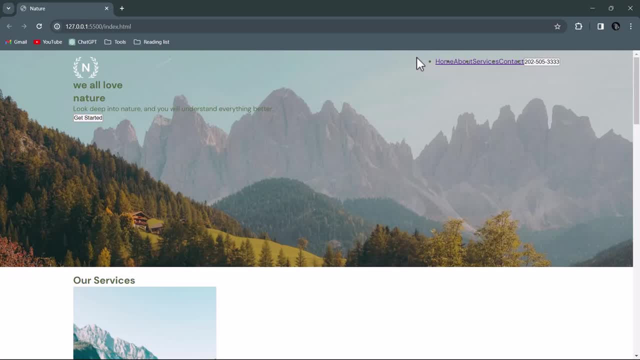 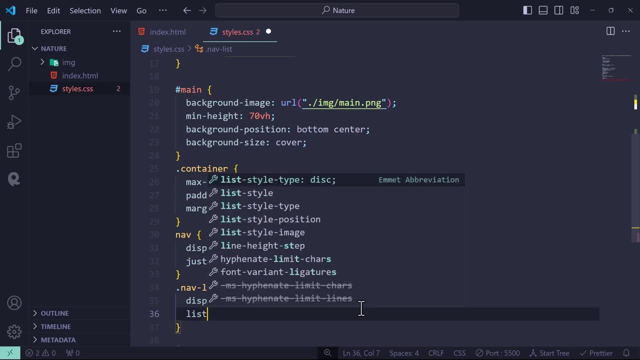 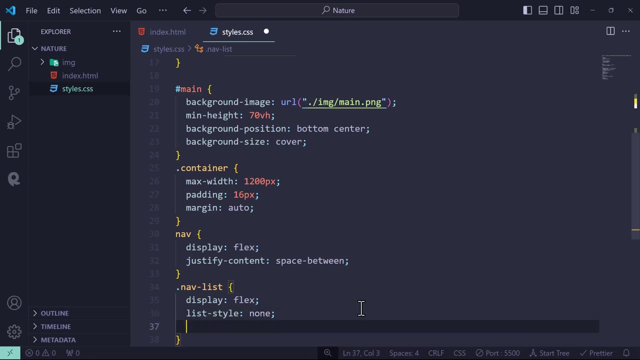 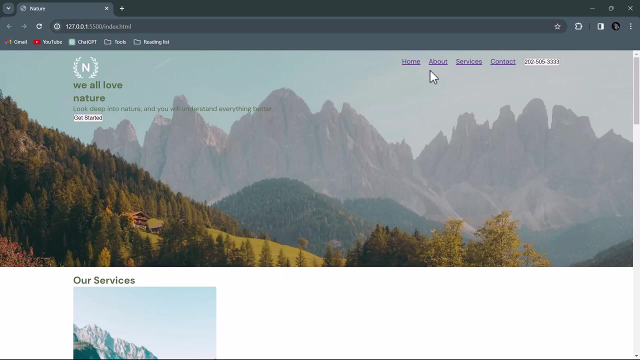 now. now these will align in your row, as you can see, and by default, all our ul's has a style. so if you remove that by using list, style none and will add a gap of 20 pixel between them, as you can see, we have the 20 pixel of gap between each of those. let's make it 28 pixel. 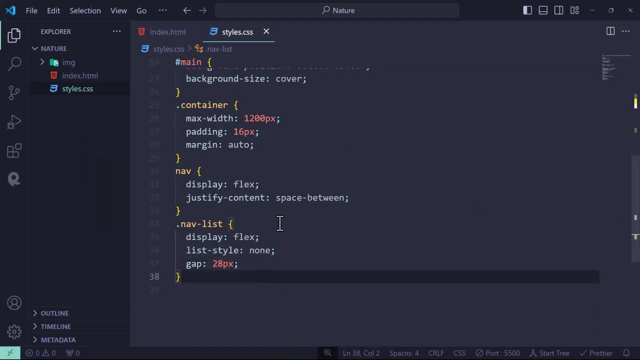 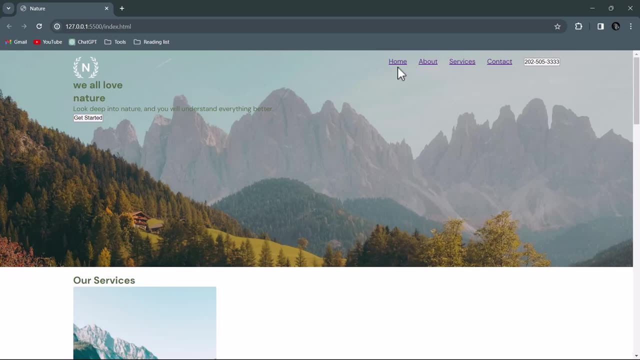 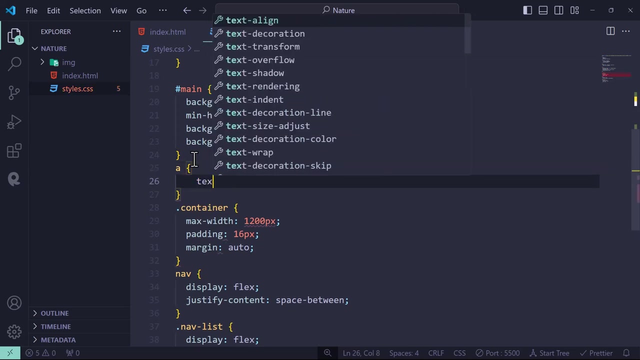 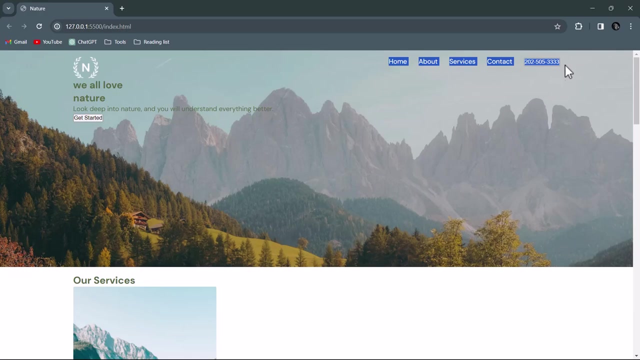 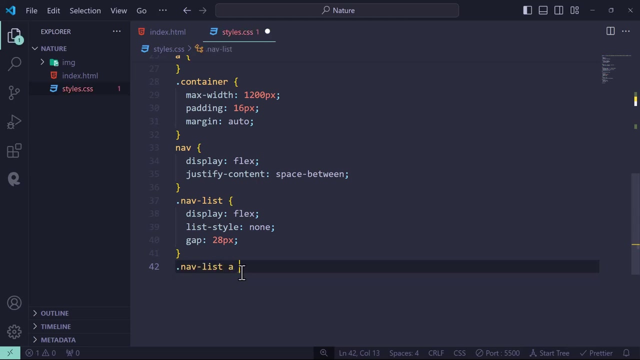 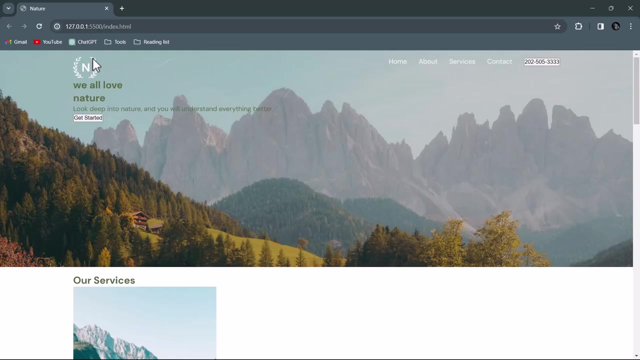 grid. now, as you can see, as we added anchor text for these nav items, by default have an underline, so for all of our anchor text, text decoration should be none, as you can see, now that underline was removed. so after that, inside nav list for the anchor tag, let's add color to white and, as you can see, this logo and is starting. 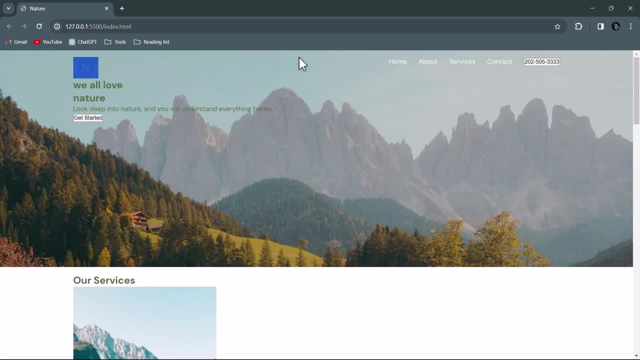 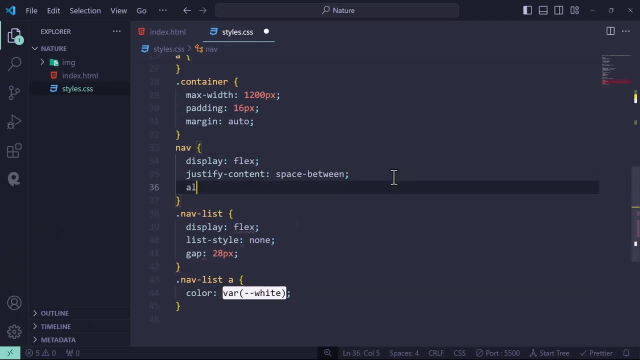 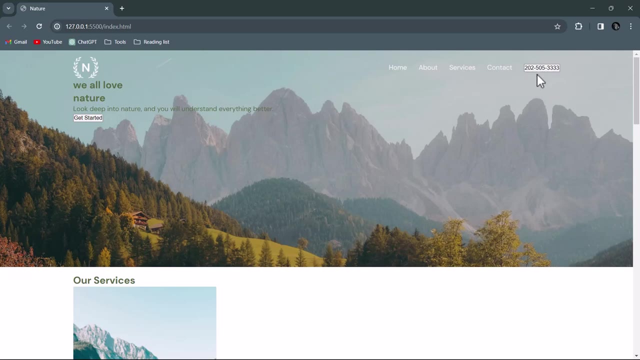 at here and this now items is also starting to the top of this logo. we want these to be in center to this logo, so to do that for the now, if you make align items center, you can see this was aligned in center. so for the button right here and all of these buttons, 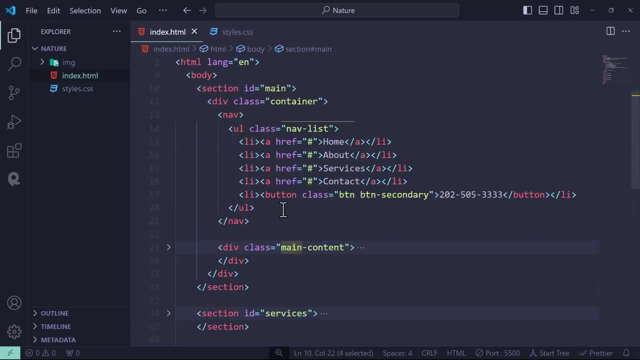 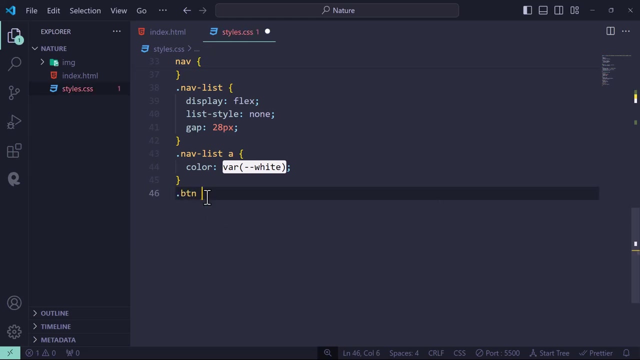 if you remember, for each of the buttons, as you can see, we have two class names: one is btn and one is btm secondary or btm primary. so by default, each of the buttons should have the styles that we applied to btn. so for the btn class name i will add padding 12 pixel. 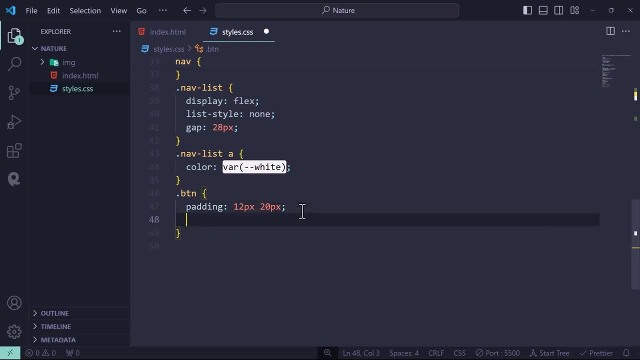 top and bottom and 20 pixel left and right. so by default i'll remove background and color to transparent and outline none and cursor pointer- as you can see when i hover on it will be pointer and i will add a border radius of 5 pixel. great, now for the btn primary. 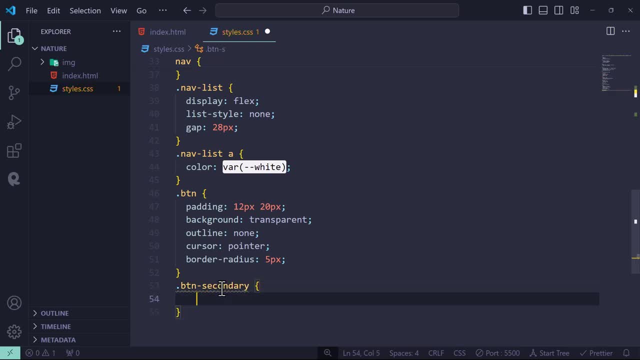 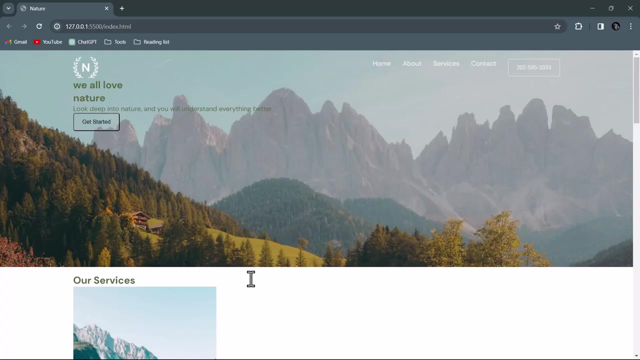 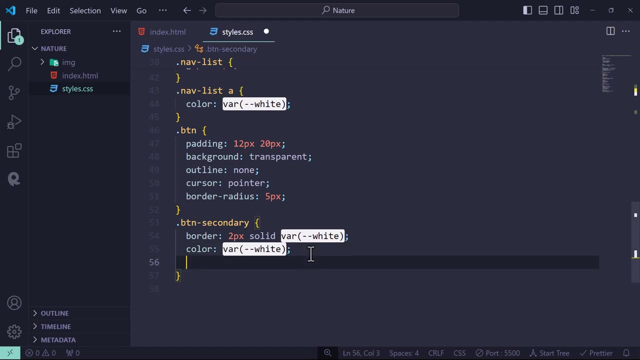 for the btm secondary. i'll add a border of 1 pixel solid of white, and the color of the text inside this button should be also white. now you can see this was in white color. let's make this to 2 pixel and for this font weight bold. you can see we have this beautiful button, so as you can. 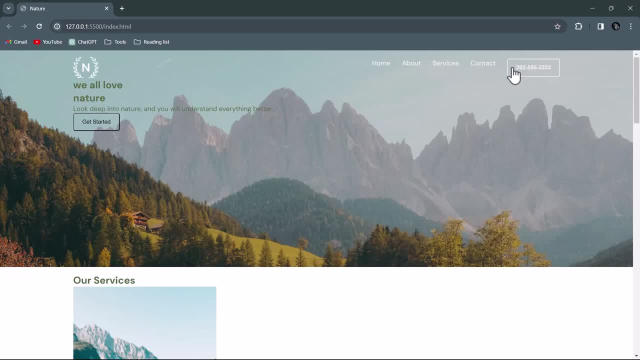 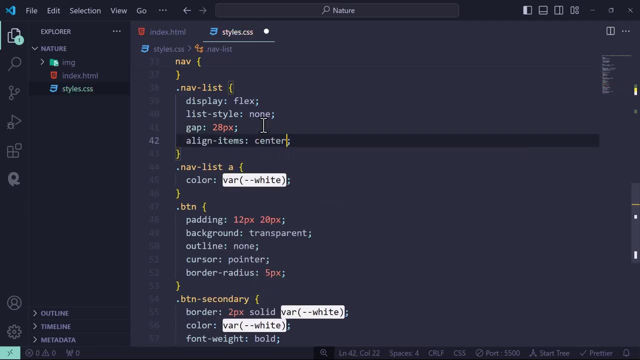 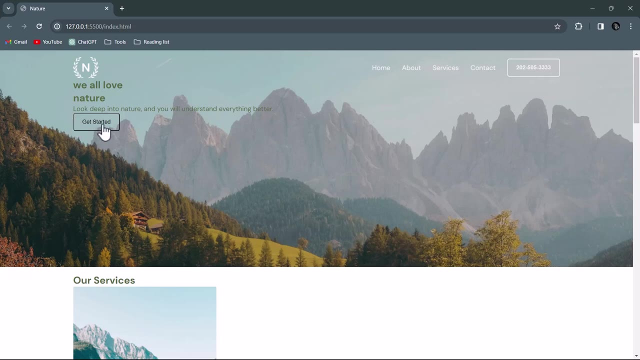 see this button is also starting at the top of this list to make these two center aligned for the now list. as we applied display flex, if you add align items to center, you can see this was aligned in center. great, now for the btn primary at the bottom right. here for the. 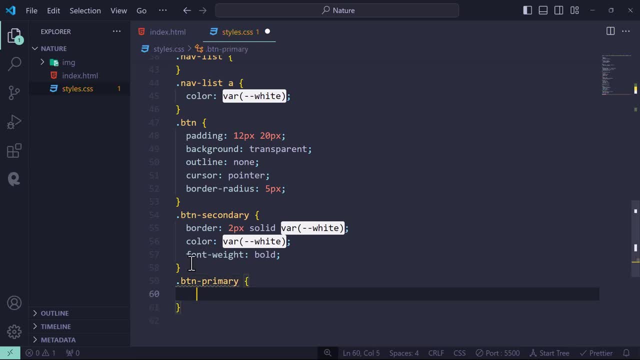 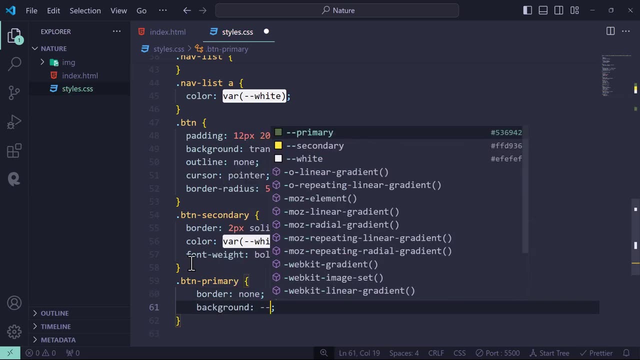 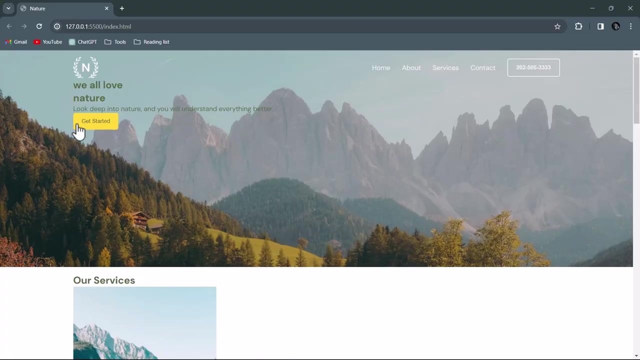 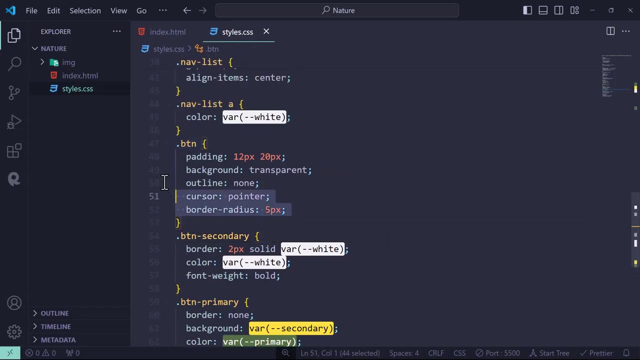 btn primary. let's make border to none and background to secondary color and color to primary. now you can see we have these beautiful buttons at here and there also. so, as you can see, with one class name, we applied all the global stylings to these buttons and as we 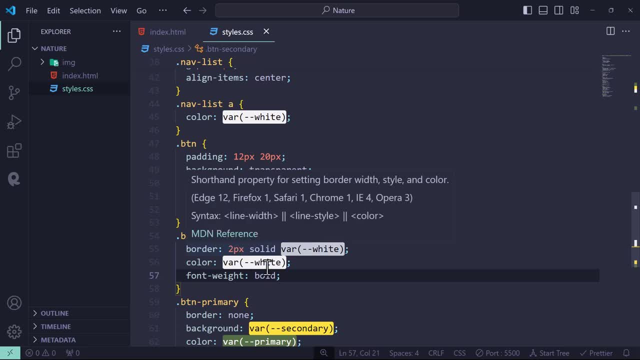 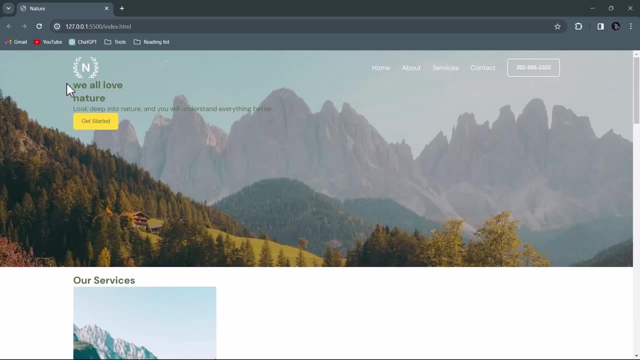 need some specific styles to some of these buttons, we can apply all the global stylings to these buttons. and as we need some specific styles to some of these buttons, we can apply these specific button. we added this extra class name of secondary and primary and we made the changes accordingly. now let's target this main content, which is this main content. 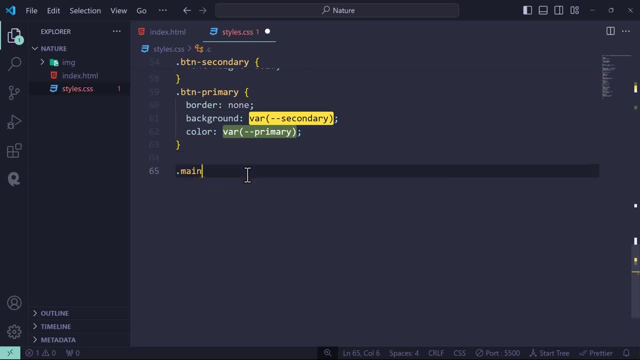 so inside CSS for the main content I will make displays flex and flex, Direction this column and align items center and justify content center and add margin. top 80px insert main content, for our entire text should be in white. you can see now these are all in white. 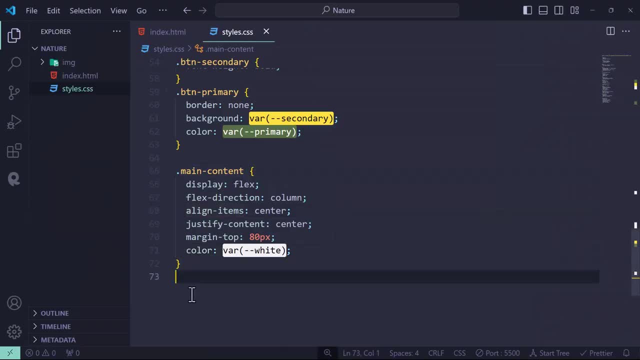 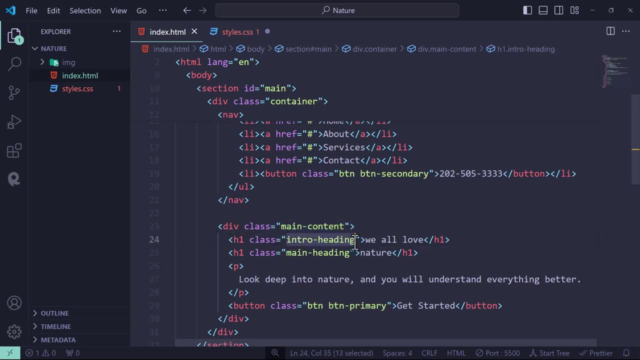 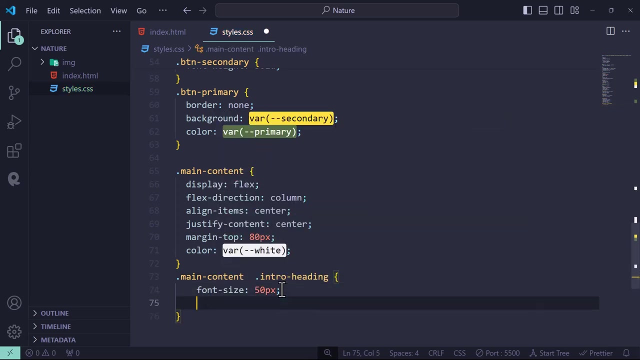 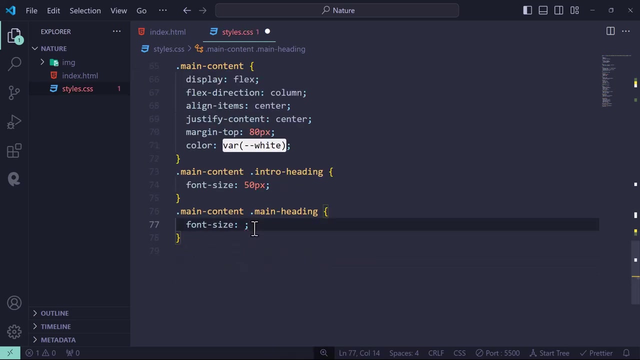 and insert main content for the h1, which is this h1 right here: intro heading: lets add font size to 50px- you can see we have 50px. and for the main heading, lets make font size to 110px and margin: top minus 20px. 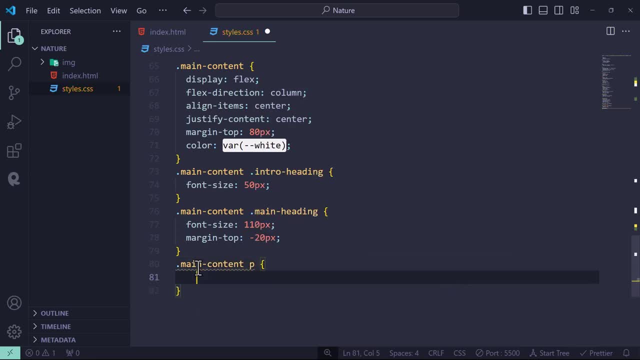 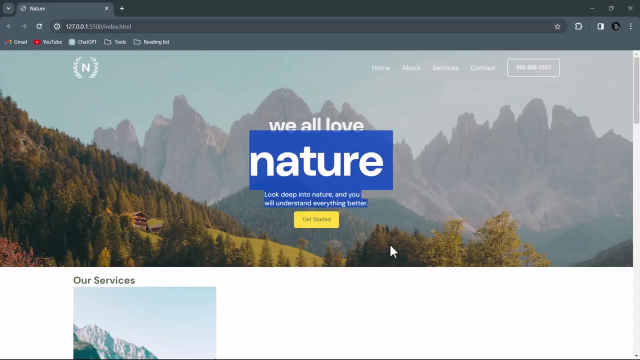 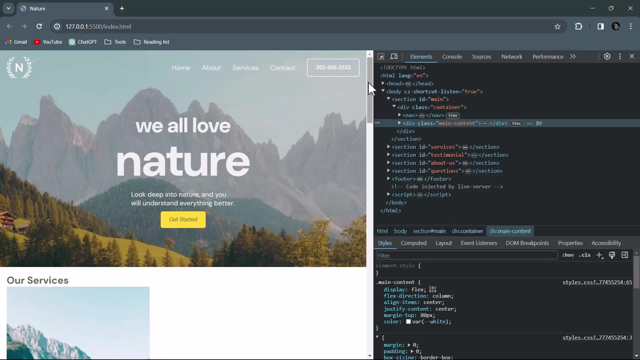 and insert main content for the p tag. lets add max width to 250px and margin bottom 10px. you can see we have this beautiful header content. now lets make this header responsive. so lets inspect this and open inside mobile browser. as you can see, this is not at all responsive. 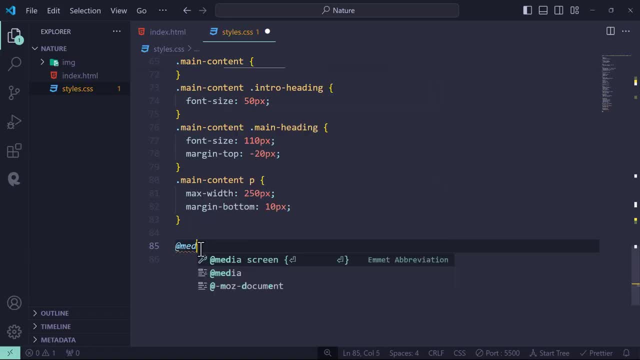 so to make it responsive, add media screen and max width of 520px, and if the screen size is less than or equal to 520px, all the styles that we gonna write here will be applied. add here for the nav list. i will write flex direction to column. 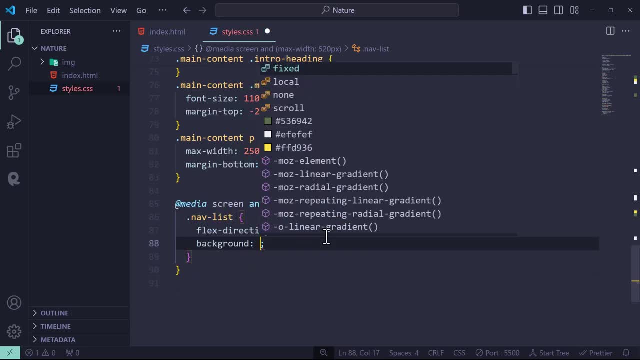 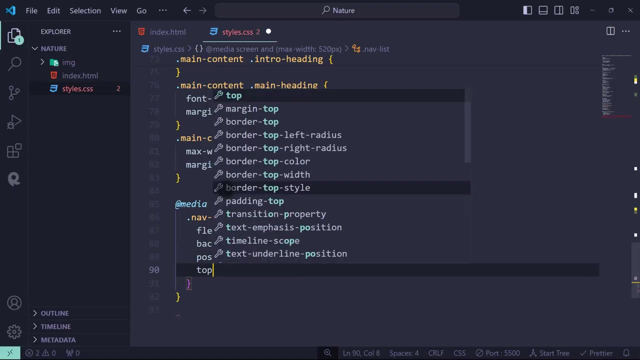 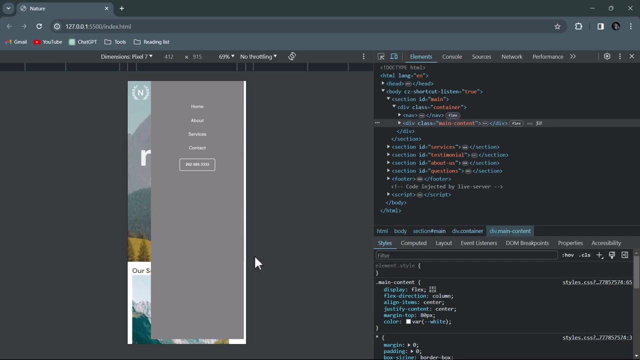 and i will add a background of grey. as you can see, we have this grey background and i will make position to absolute and top 0 and right 0 and width 80% and height 100vh, padding top of 80px and inside this nav list. 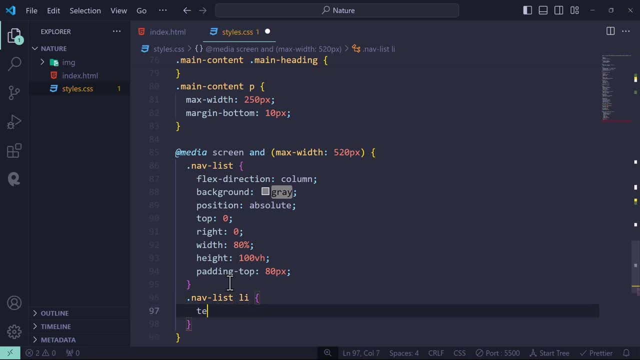 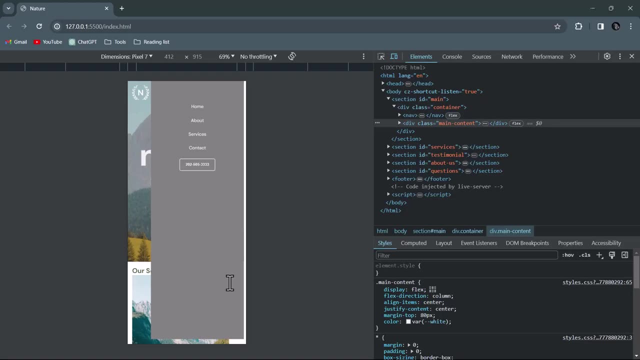 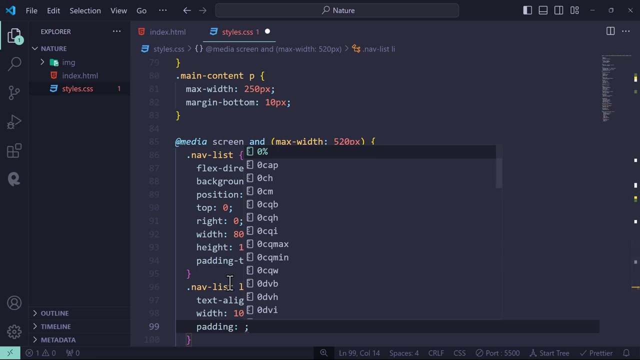 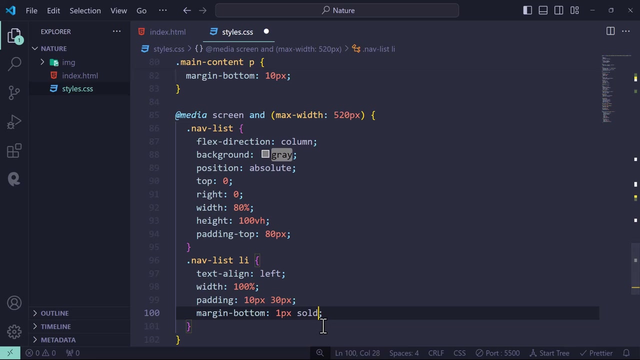 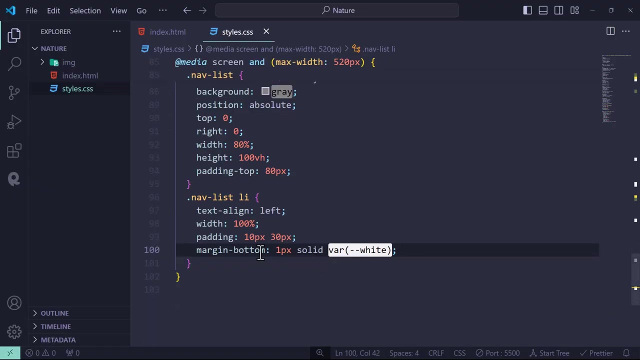 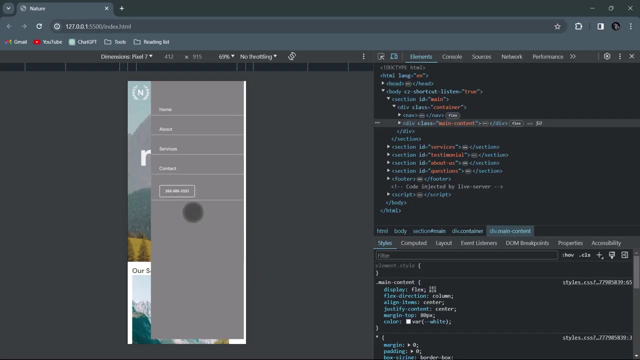 for each ally. i will add text align to left and width 100% and padding top and bottom 10px and left and right 30px, and i will add margin bottom of 1px solid of white. this should be border bottom, as you can see. 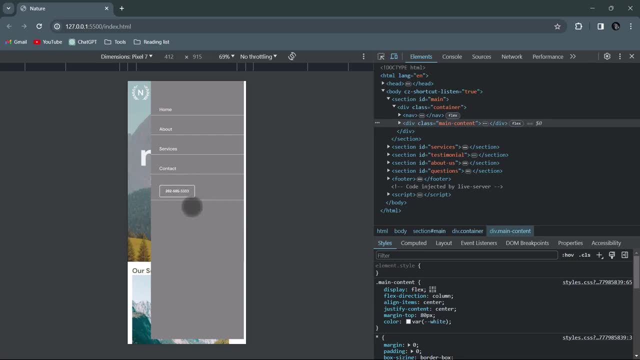 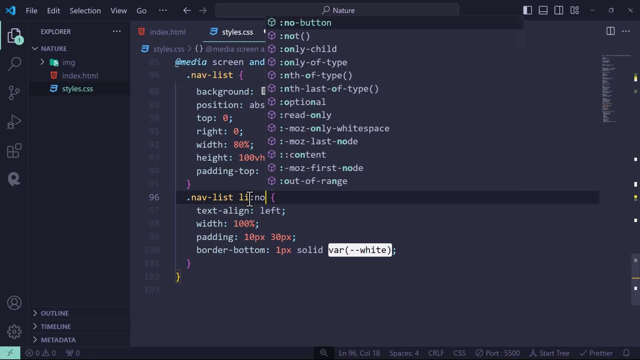 this was applying the border to this button. also. we don't want this border for this button. so to do that for this, we have sss property called not for, which we don't want that. we don't want that for last child. if we apply last child. 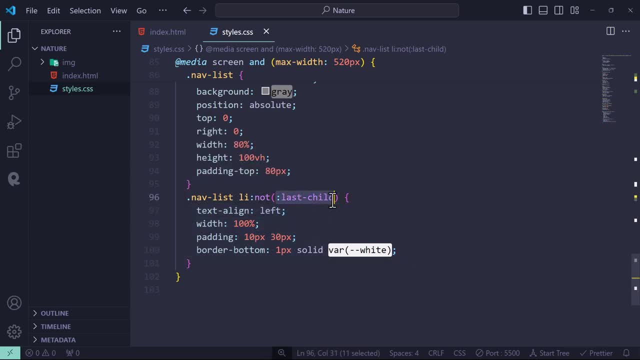 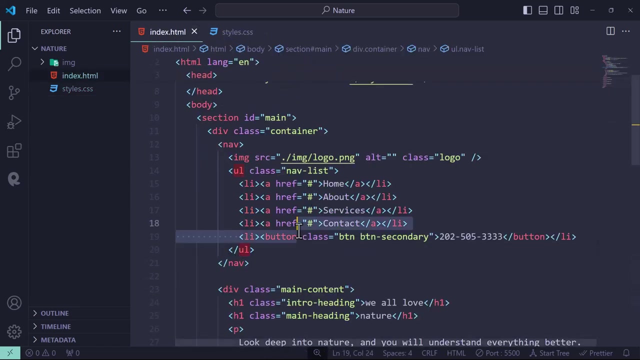 so all these styles for the last child. it won't apply. so inside these allies this button is the last child, so this border is not applying to this button. so now we should add a button here like a menu toggle, so to add that inside the ul or after the ul. 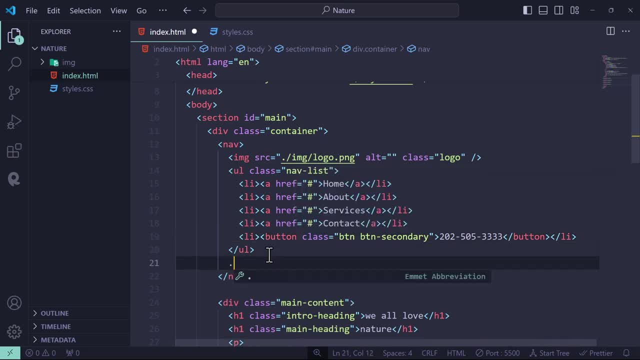 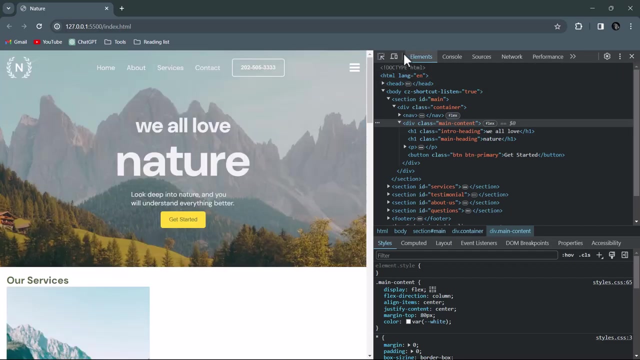 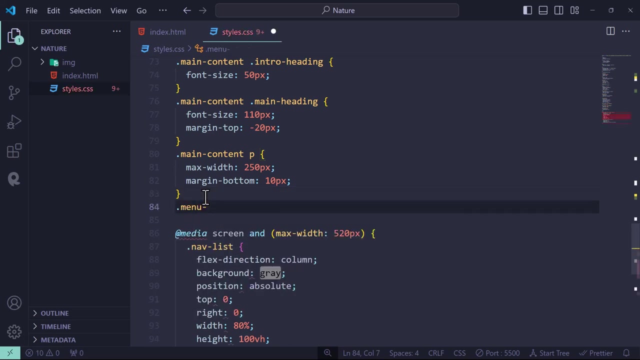 let's add a div with a class name of an image, with a class name of menu btn, in which inside images menu, dot, svg. as you can see, we have this menu button. so for this menu button, insert css at the top right here for the menu button. 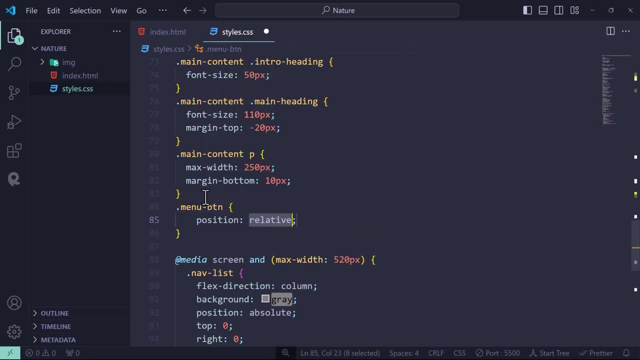 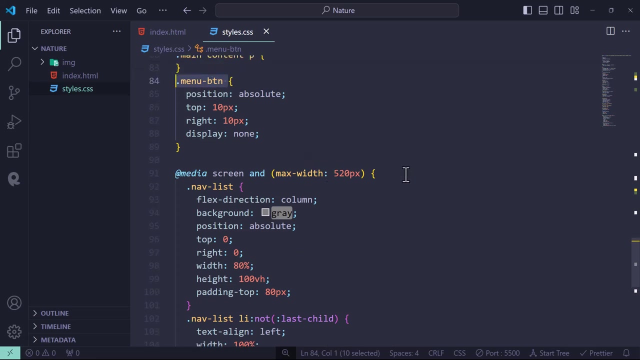 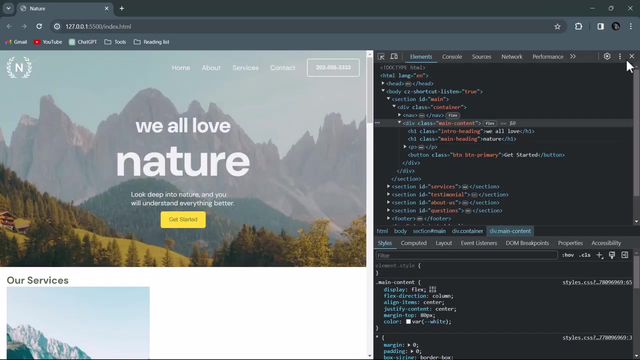 let's make position as absolute and top 10px and right 10px and this should be hidden display. none on desktop. when it was inside mobile, have to make display block. as you can see, inside desktop we don't have that button, whereas in mobile we have that button. 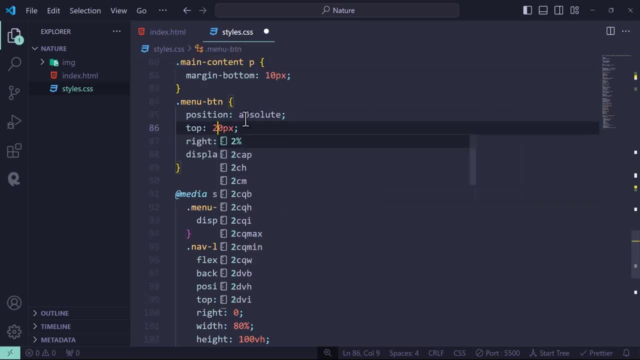 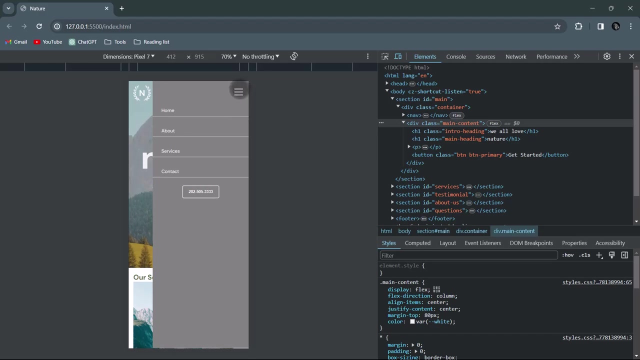 so let's make it top 20px and right 20px, so that we have some extra space. let's add a width of 30px. great. now, when we click on this button, we have to hide this and when we click again, we have to show this. 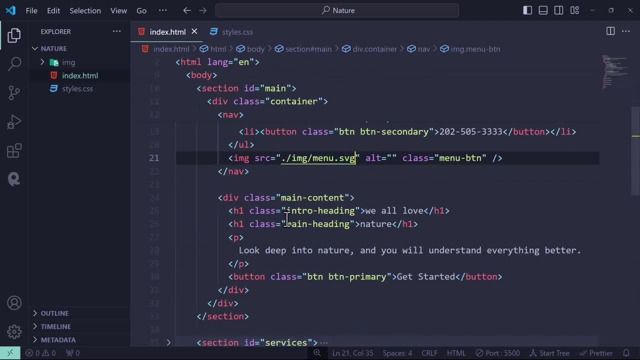 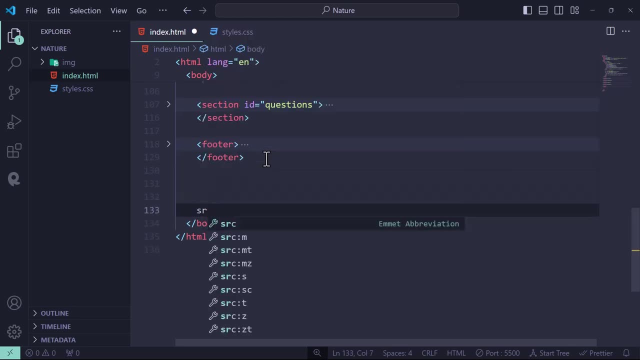 so to do that, let's open the indexhtml file and at the bottom, right here, before closing body tag, let's write a script. if you don't know javascript, just follow along. you will able to achieve this effect inside this script. we have to write a variable called 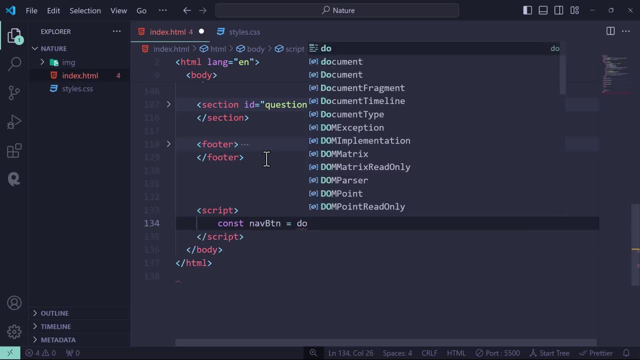 now button which should be inside our document dot query selector. this should be menu btn, which is that button. so and we have to get our now list. this should be inside document dot query selector. this is our now list, so when we click on that now button. so for the now button. 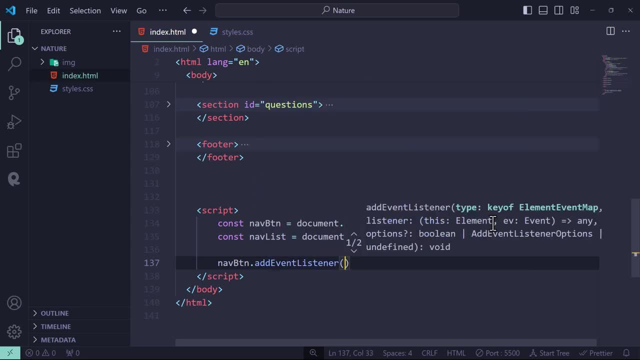 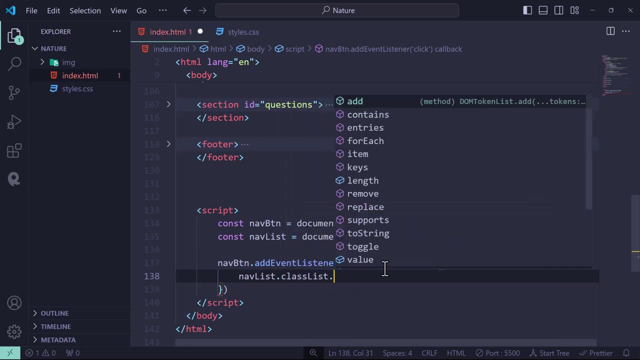 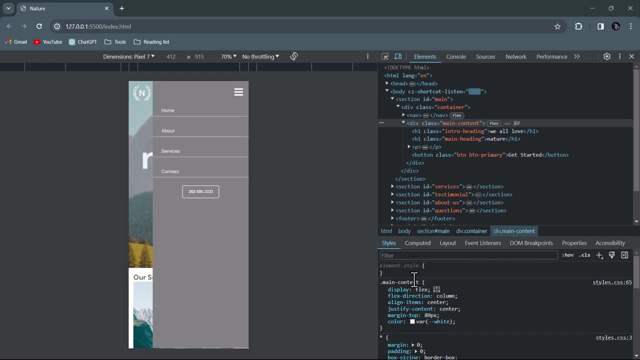 we will add a event listener which should be click. so whenever we click on this now button, we have to run a function. inside that function we have to define: for the now list dot, class list dot toggle we should add a class name called active. so what this will do is that 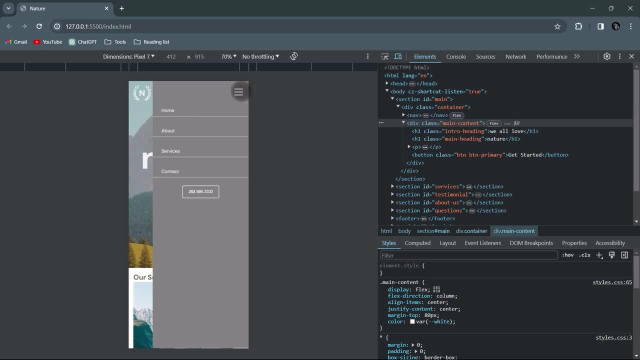 as you can see whenever I click on this. you can see whenever I click on this menu button, this active class name is toggling for the now list. you can see we have active. when I click again, we don't have that active. so whenever this class has an active 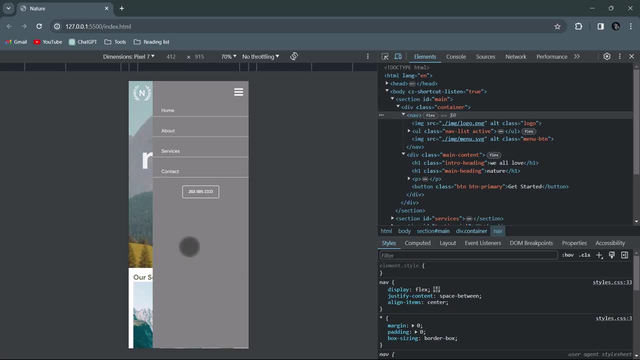 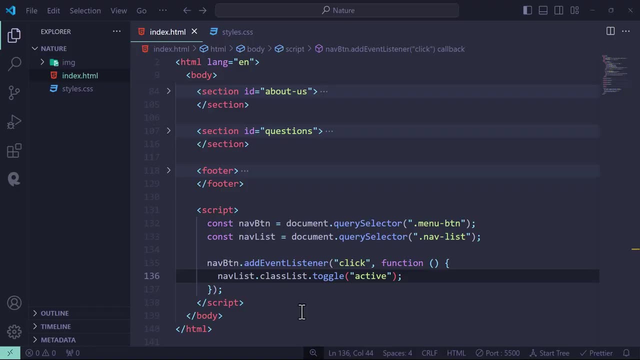 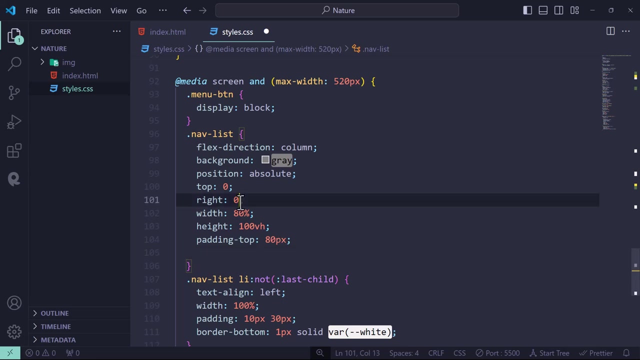 we have to show this, this side bar. this now links inside this side bar. whenever we don't have that active link, we have to hide that. so to do that by default, we have to make write to minus 900px so that it will. it will go out of the screen. 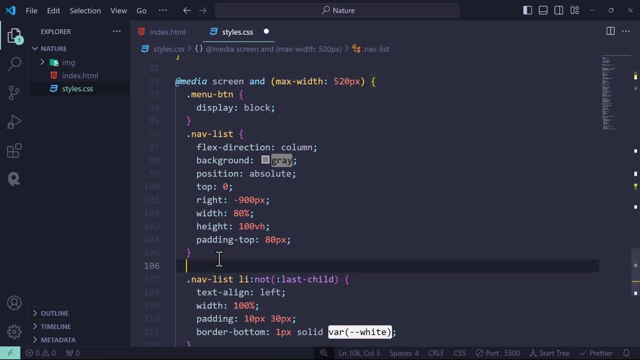 so whenever this now list has in class name of active, so we have to make sure there is no space between this now list and this active. so whenever this now list has also has in class name of active, we have to make write zero so as you can see. 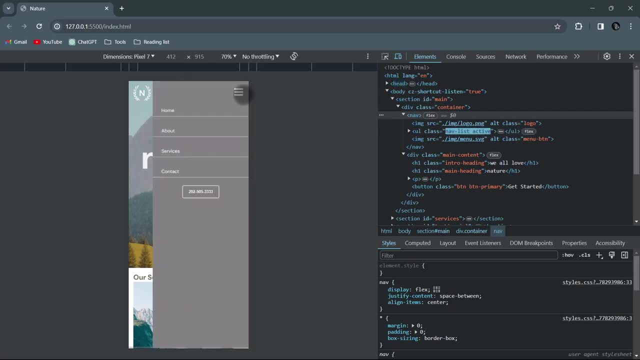 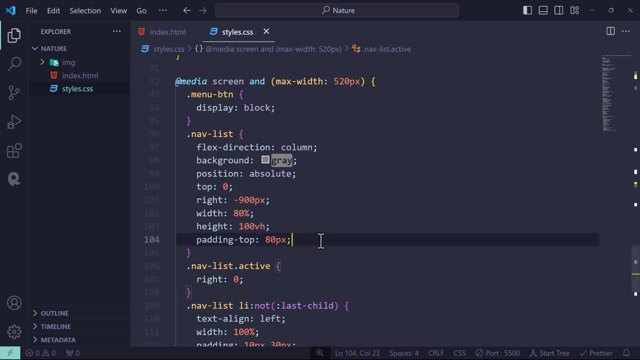 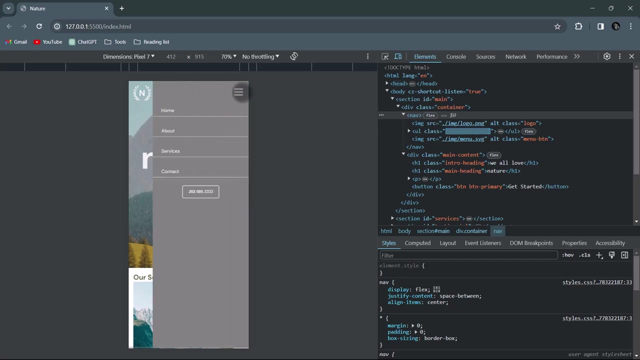 we have this beautiful navigation menu so we need a smooth effect to this. so to add that for the now list, if you add transition of 0.3 seconds, for all 0.3 seconds is you can see this smooth animation. great, right, let's move on to our next section. 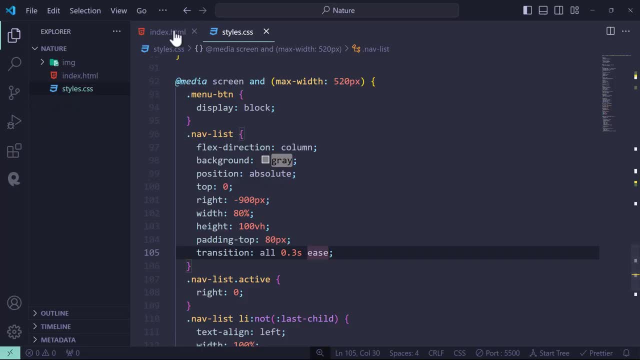 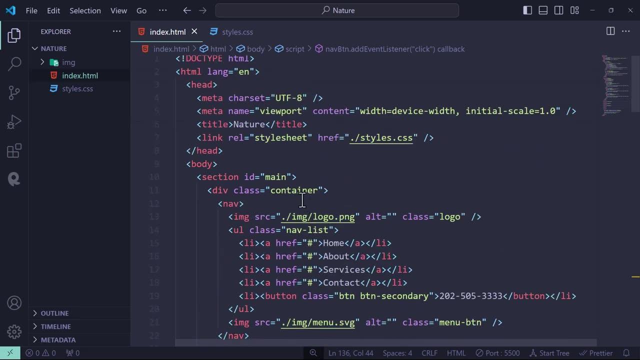 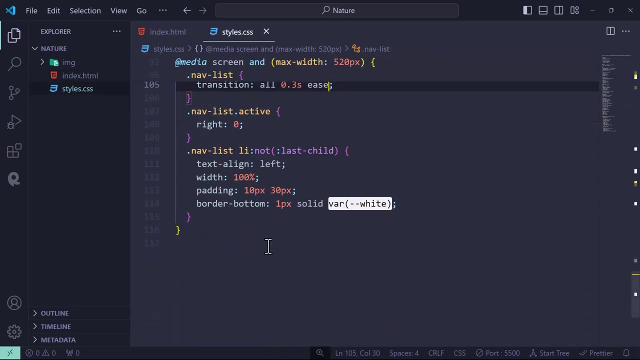 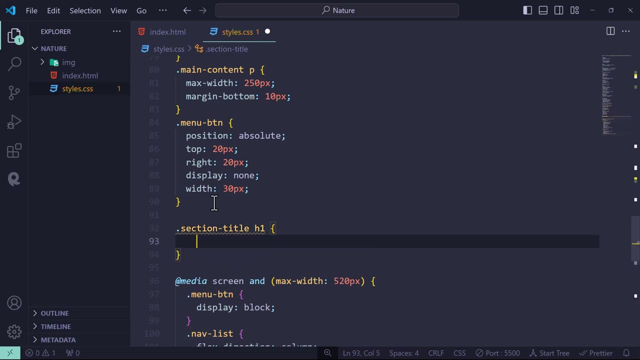 which is our services. so, as you can see and if you remember, inside services section, we have this section title. so at top right here, inside section title for the h1, let's make font size 250px and text align center. and inside section title for the line. 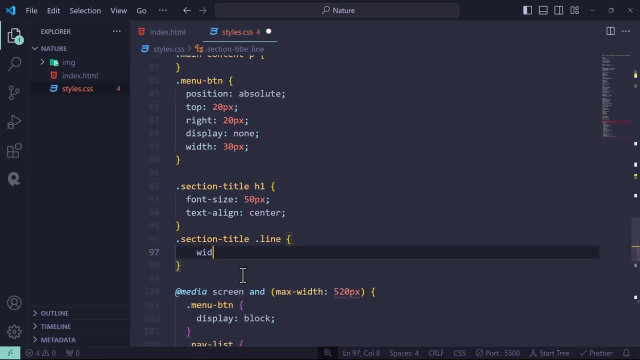 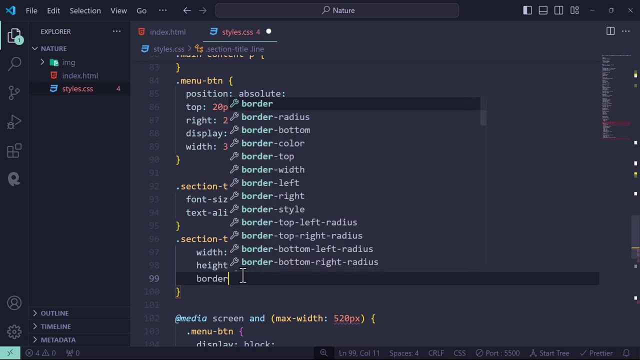 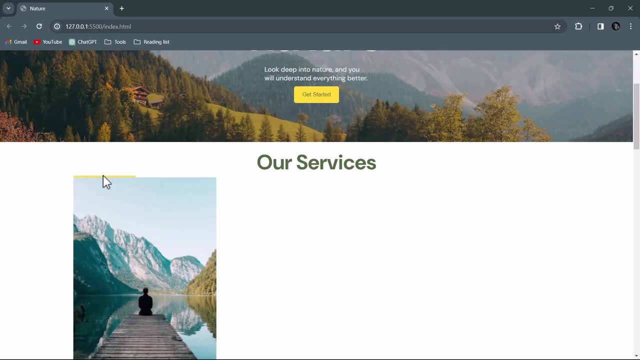 let's make a width of 150px and a height of 4px and border radius of 10px. this should, as a background of secondary. you can see we have this line right here and for this, if you add margin, auto that will come to center. 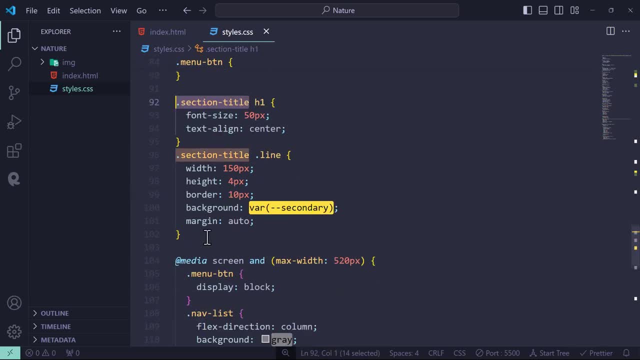 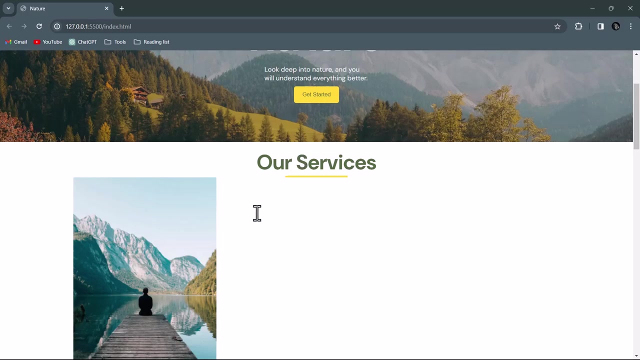 great right now for the section title. if you add margin auto, that will come to center. great now. as you can see, for each of each of our section we should have a space between each of those sections below this container. for this section I will add margin top and bottom. 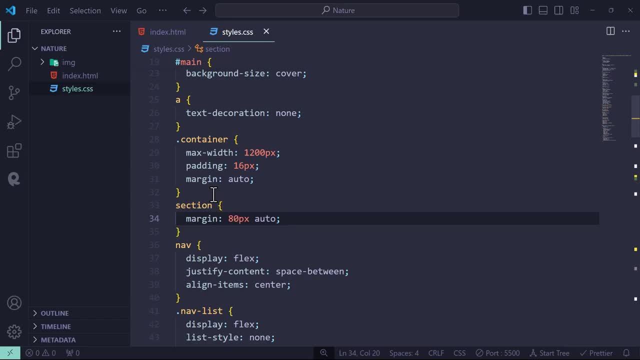 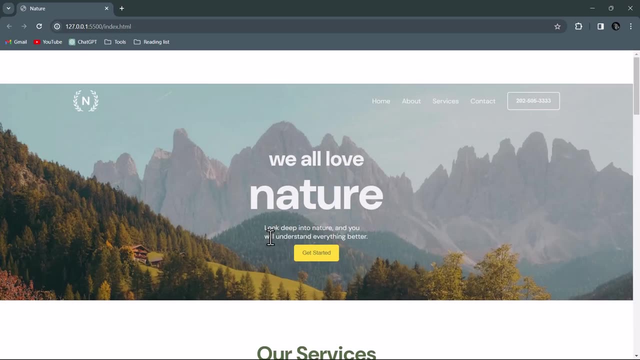 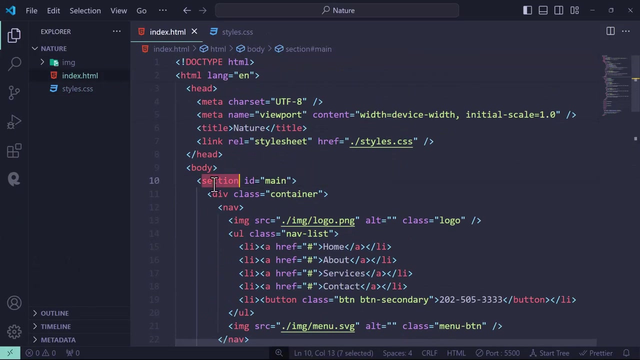 80px and left and right auto. now you can see each of our sections has minimum space of 60px and by default it was applying to our header section, main section also. so instead of giving it section, I will rename it to div so that we don't get the 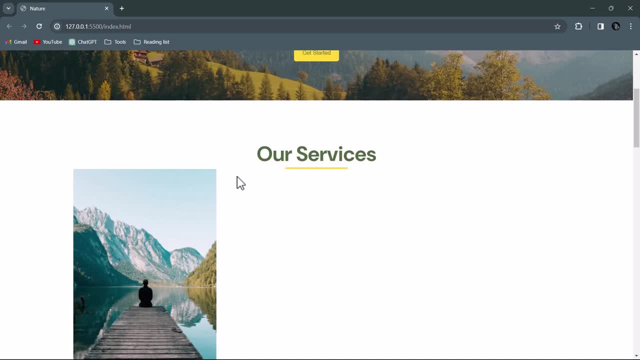 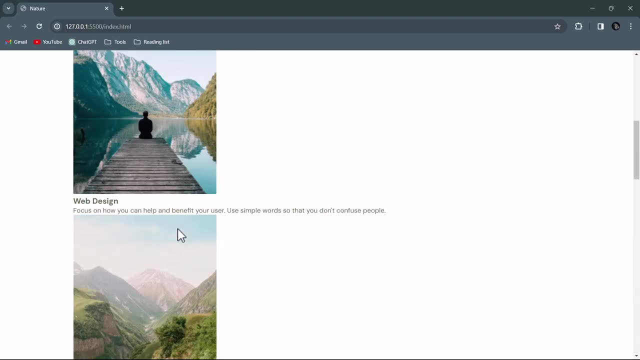 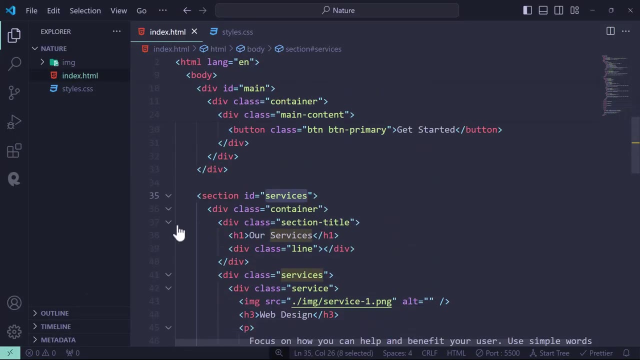 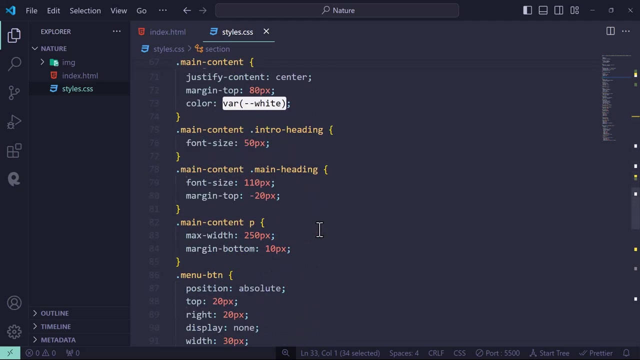 styles to our main section. except that main section, all of our, all of our section will have a space of 60px on top and bottom. so inside the services section, after the section title, we have a class name of services, the bottom right here for the services. 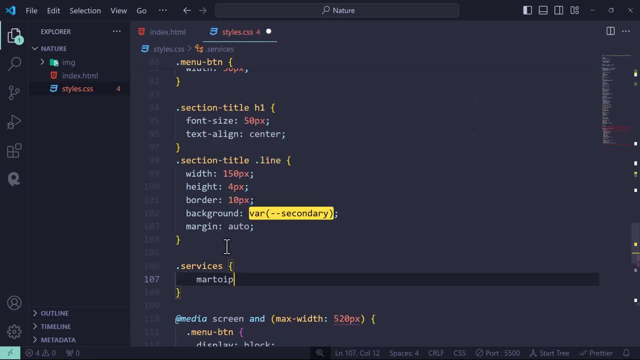 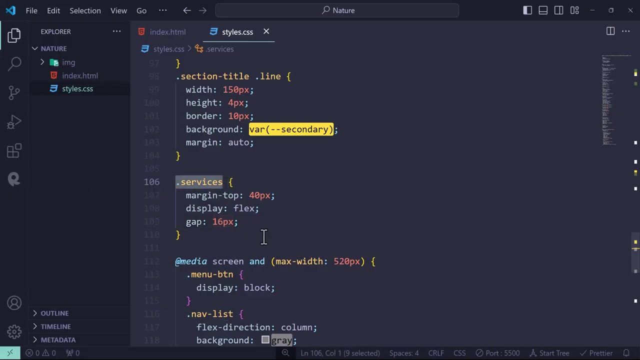 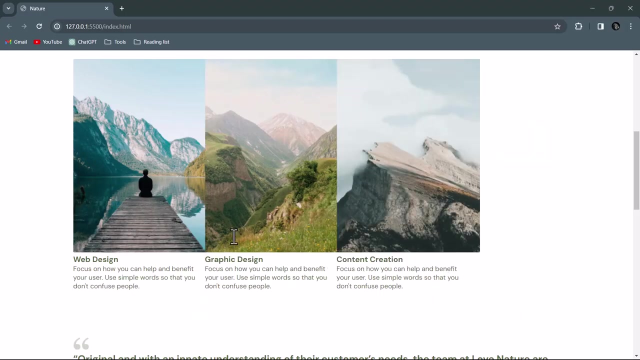 in which we have all of our services. I will add margin, top 40px, and I will add display. let's add a gap of 16px between each of those and inside services. for each service, I will add a width of 300px and, as you can see, 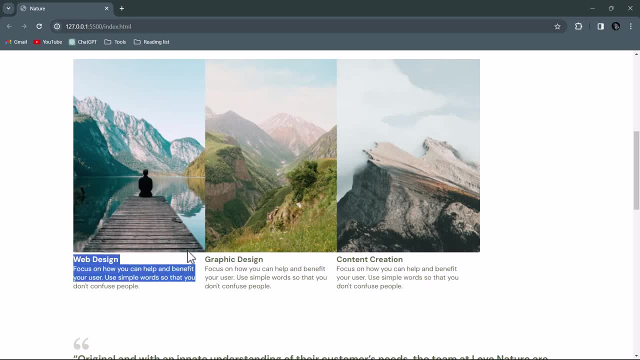 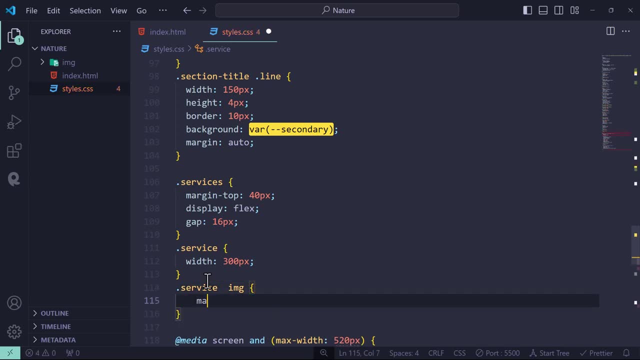 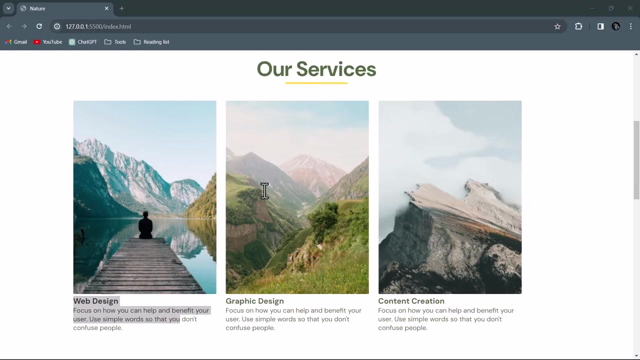 our image is overflowing more than 300px. so to remove that overflowing inside service: for the image, let's make max width 200%. so that it won't overflow, let's make this 350px. and for the services, if you make justify content center, this will be aligned. 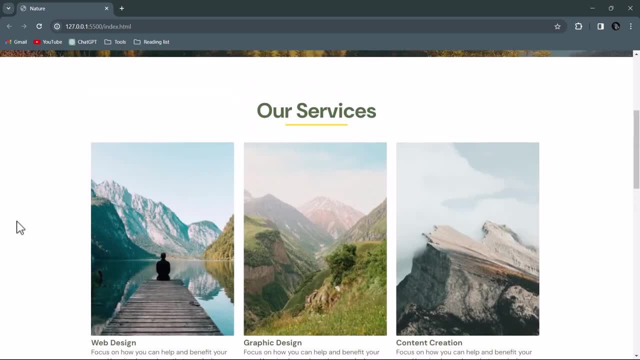 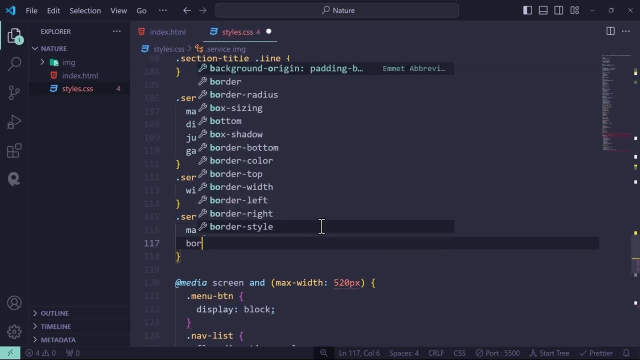 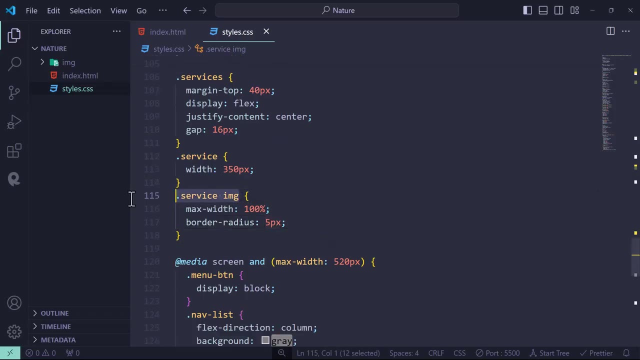 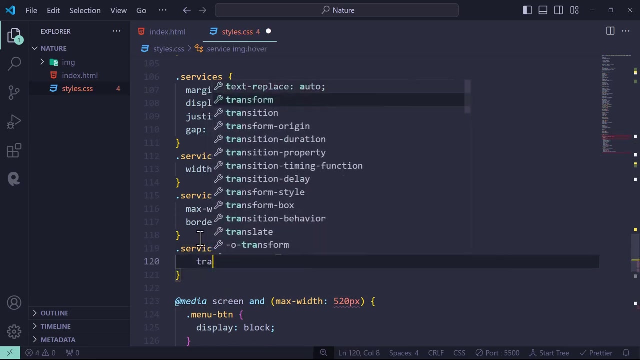 in center and whenever we hover on this image, we want a smooth zoom in effect. so for that, for this image, let's add some border radius of 5px, and whenever we hover on this image, I will make transform scale 1.2 and I will add 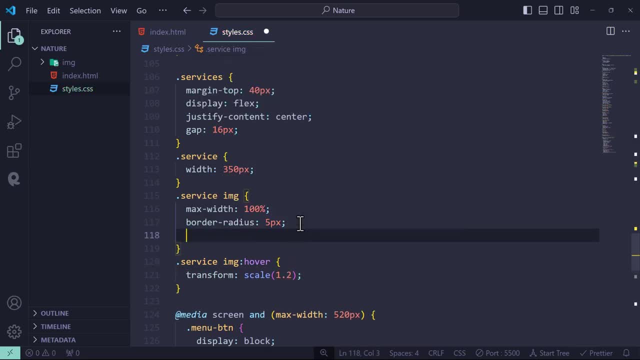 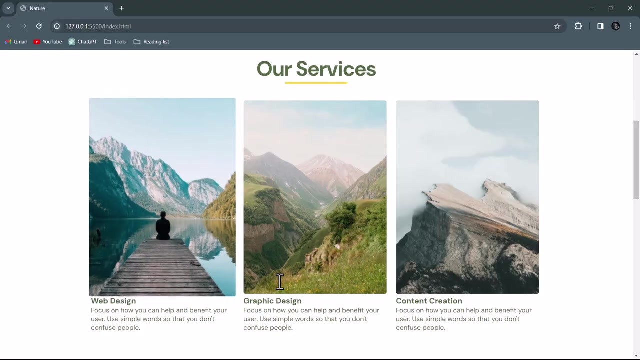 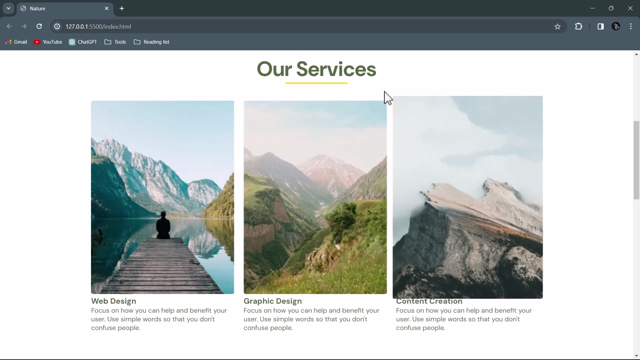 transition function for the transform, for the transform, for the transform property: 0.3 seconds of each. here you see, you can make 1.05. great, now let's try. we will set this prob like: let's see if this is responsive or not. this is not at all responsive, so to make. 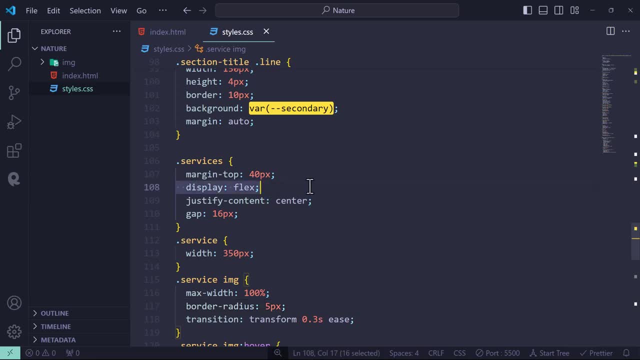 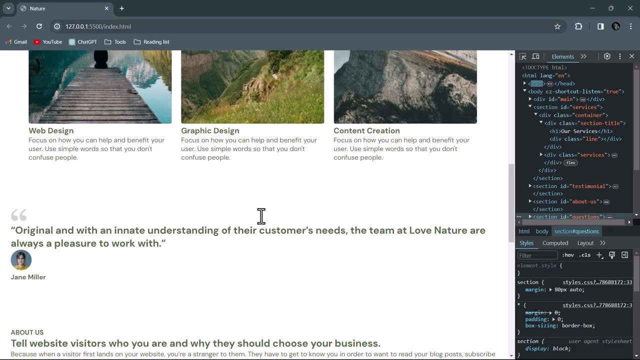 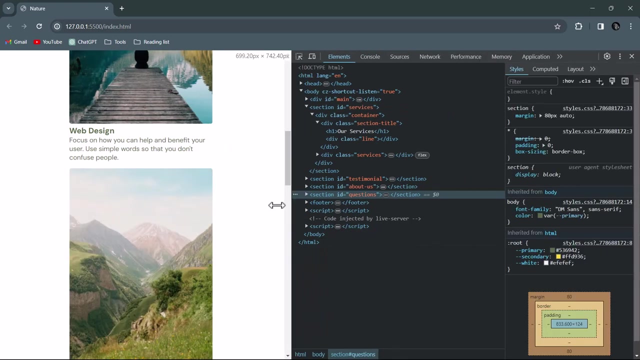 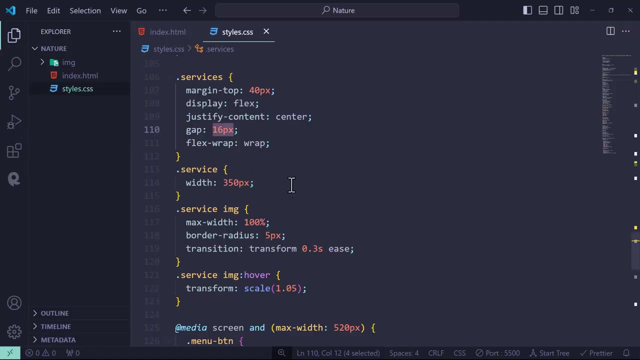 it responsive. to make it responsive, if you apply display flex and each of the style has a fixed width, if you make flex wrap as wrap whenever there is not enough space for each of the styles, that will come down, as you can see, inside the inside the mobile. now let's style our testimonial section. if you remember, we 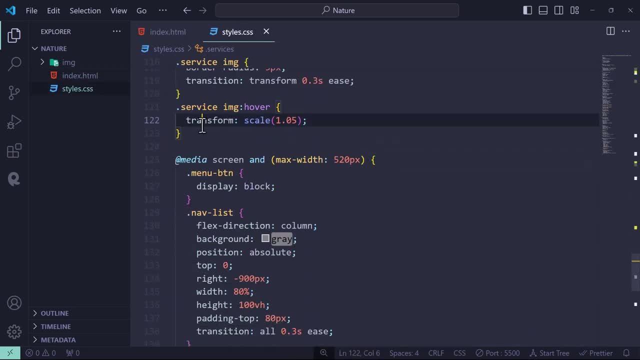 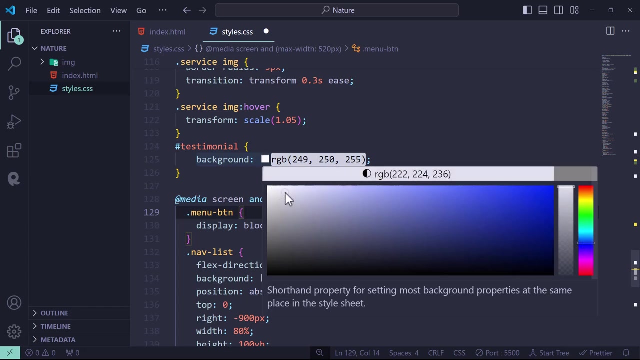 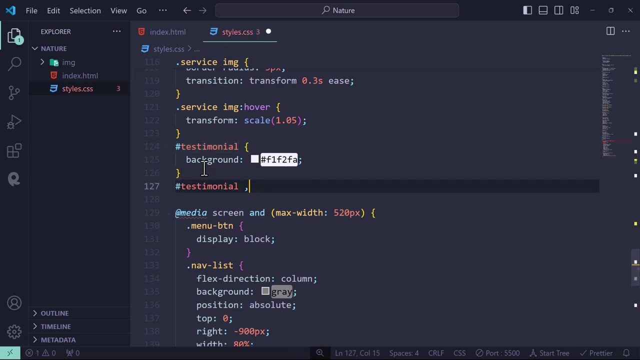 have this and I we have this ID called testimonial. at here for the testimonial section we have a background of gray color. let's change this to something like this. yeah, and inside this testimonial section we have the container. as you can see, inside the testimonial section we have the container. only for the container. 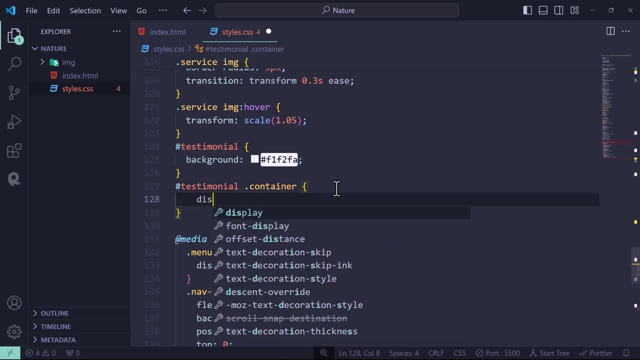 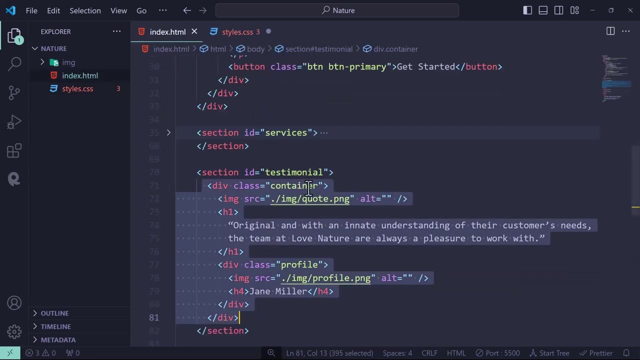 that was inside this testimonial. we make display flex and flex direction column and align items center and max width to 500 pixel and a gap of 16 pixel between each of the elements and inside this testimonial container we have. inside this testimonial we have profile which 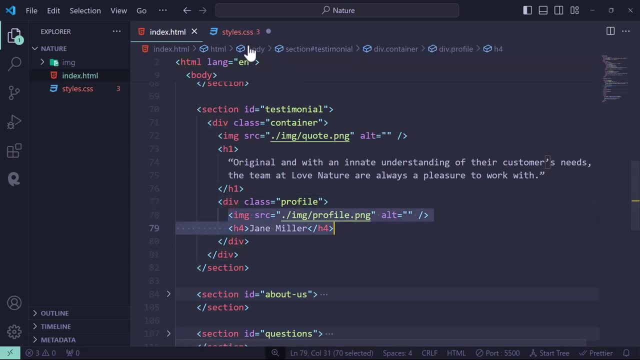 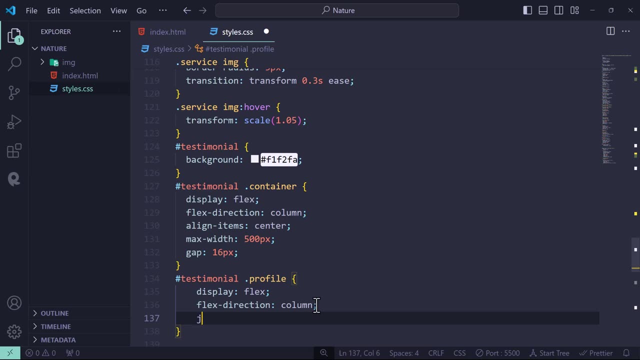 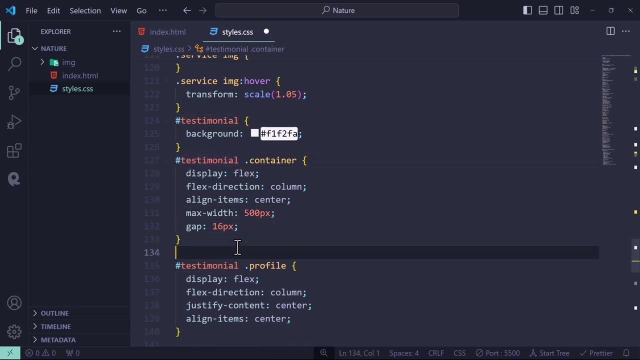 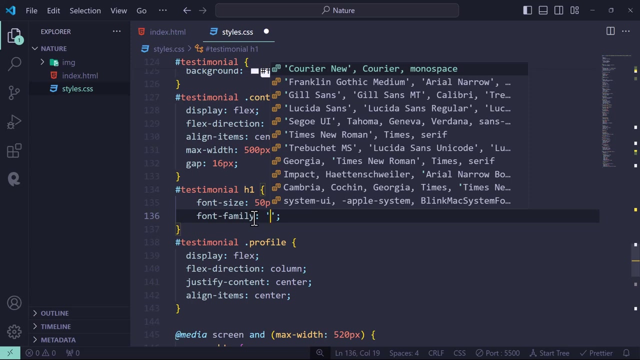 is this profile right here in which we have the image and the title. let's make display flex and flex direction column and justify content center and align items center and for inside testimonial for the H1. let's make font size to 50 pixel and font family to forum and as a fallback. 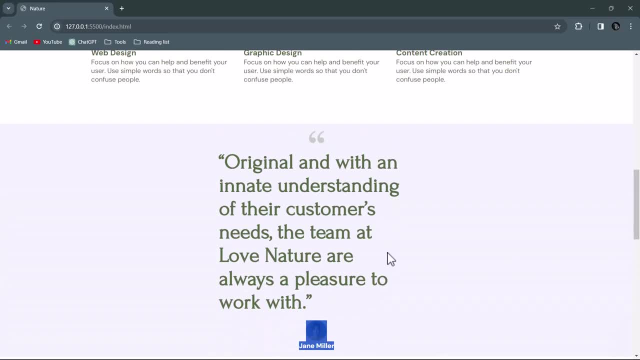 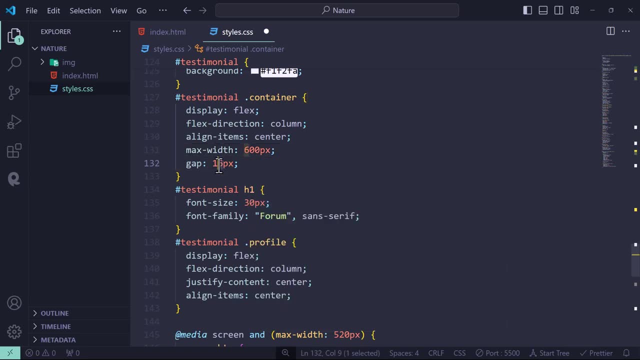 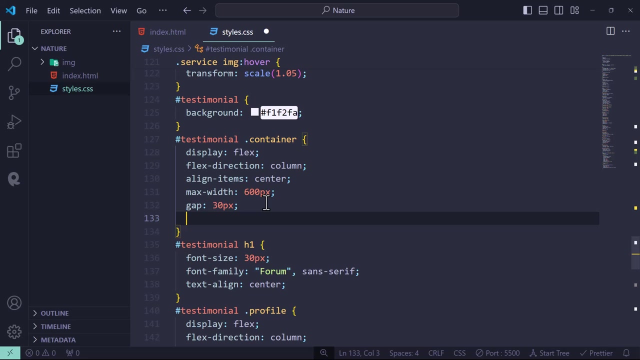 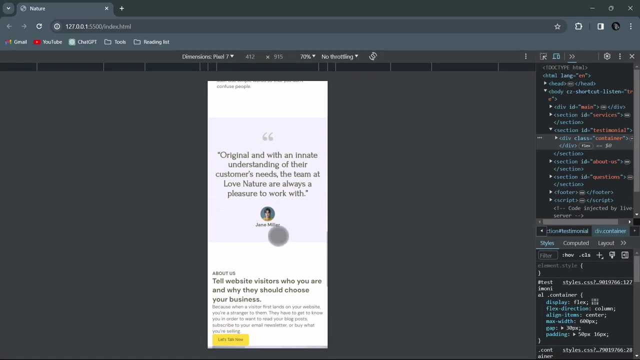 sans-serif. let's make this 600 pixel and the gap to the 30 pixel, and for the H1 text align center and for this container let's add padding: 50 pixel top and bottom and 16 pixel left and right. I can see our beautiful testimonial section. let's open this inside mobile, as you can see at. 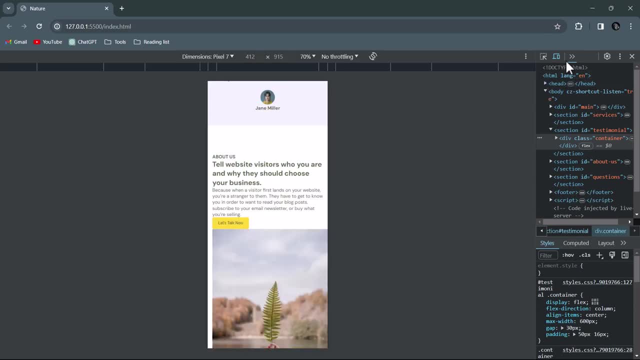 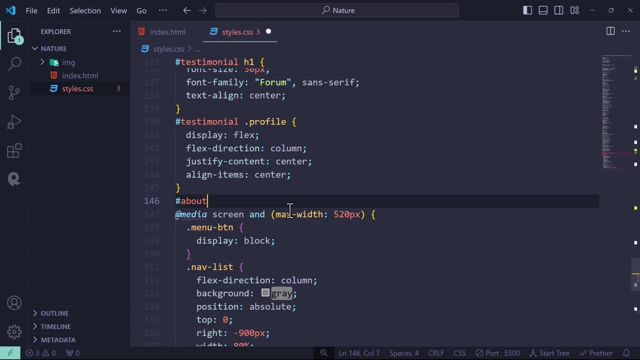 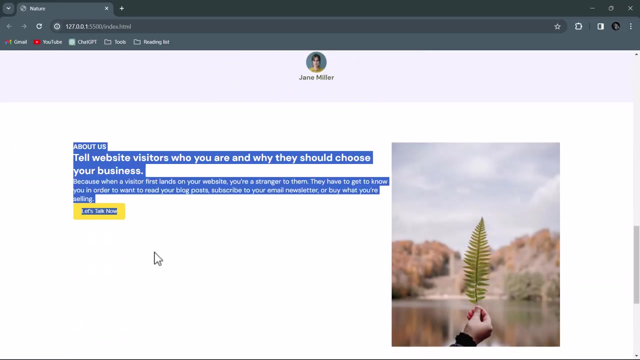 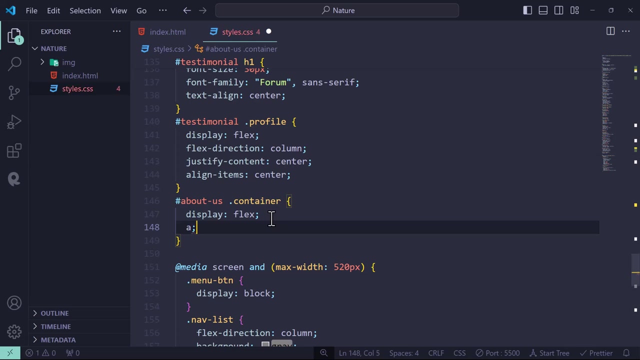 here also, it was completely responsive. now let's style about our section. so inside about us, we have the container for that. let's make display as flex. now you can see this content and this image is in your row. so inside this, let's make a line item. 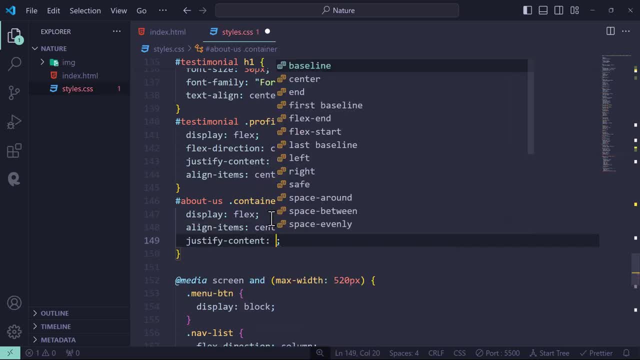 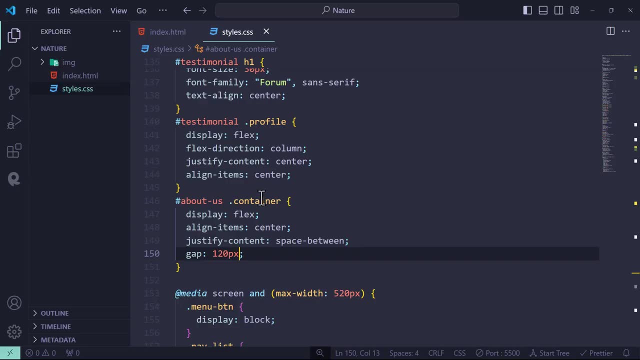 receive the value ofetta level slots are going home style. next section, from right and left, bringing which we add 4 elements to center and justify content, space between and a gap of 120 pixel and inside this container for the about content. let's make max width to 600 pixel to 500 pixel. 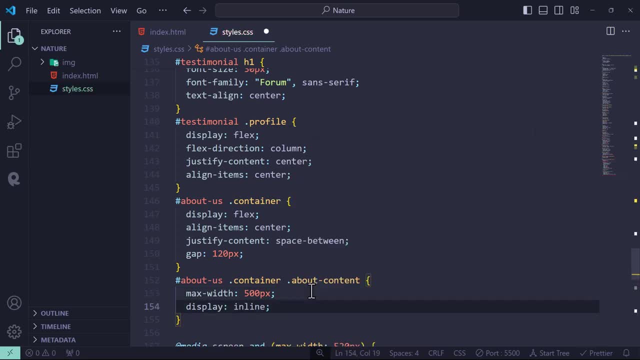 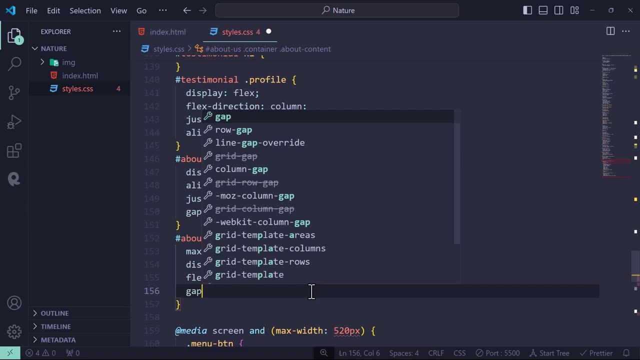 let's make max width to 600 pixel to 500 pixel. first is the medium of the luminanceteck. hereb voor thee. we need another O人ik app to select this element. let's make max width to Vivian tone ca" display flex and flex direction column, and we should, we should have a gap of 16. 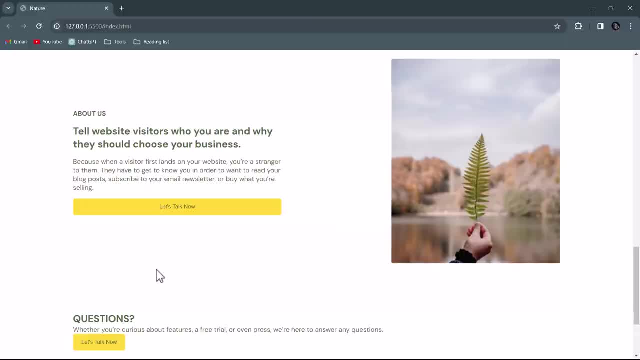 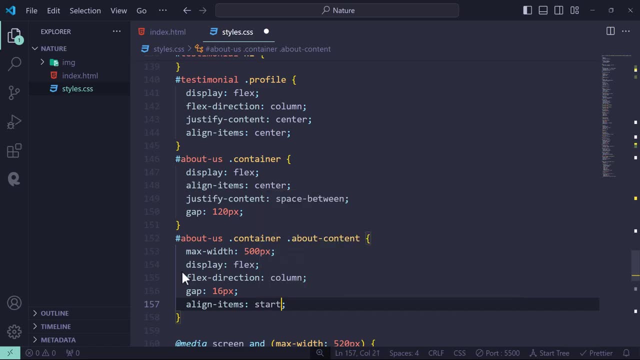 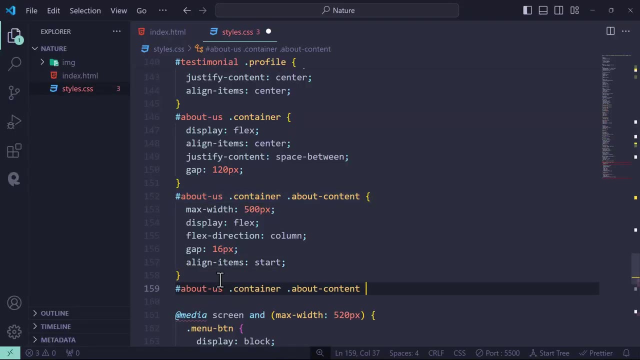 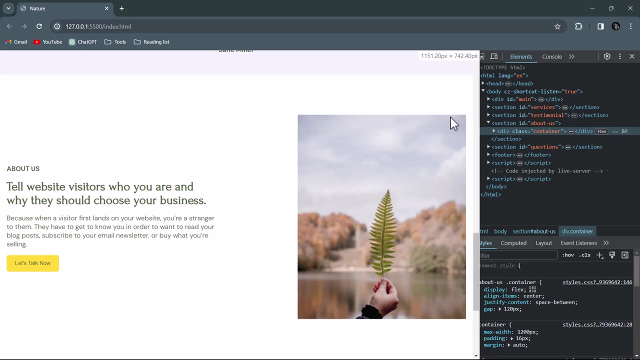 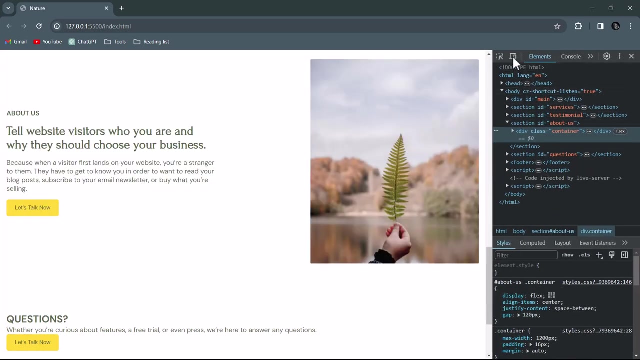 pixel and align items start and inside this about content. for the h1 we have the font family of forum and as a fallback, Sancerive and font size, the pixel. you can see this was responsible till tablet, but when in mobile this is not at all responsive. so to make this response to inside mobile. 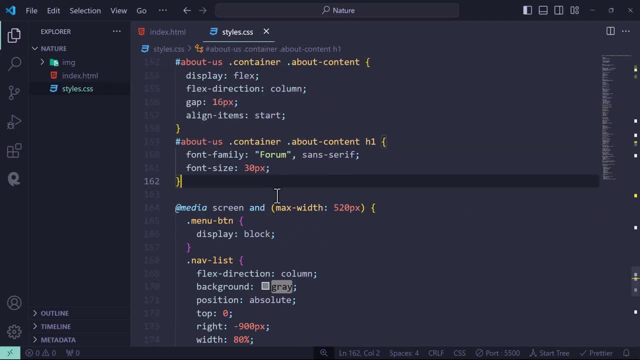 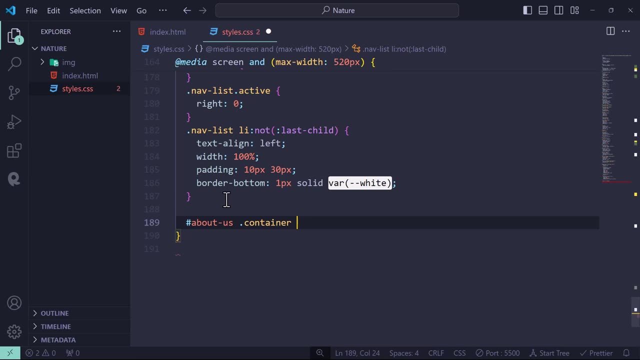 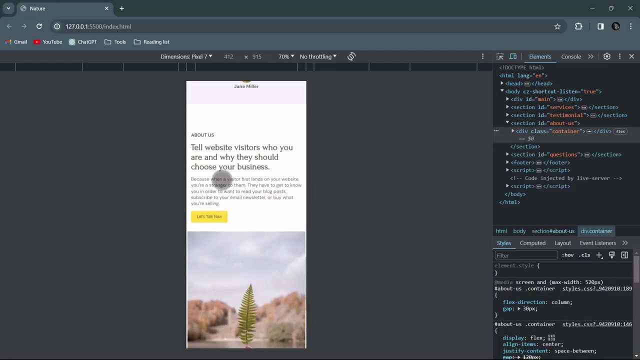 for the about us count container inside the media query and the bottom right here. let's make flex direction to column and make the gap to 30 pixel so that have less space. you can see we have this beautiful responsive water section also now. let's. now let's style our question section, which is this: questions you can. 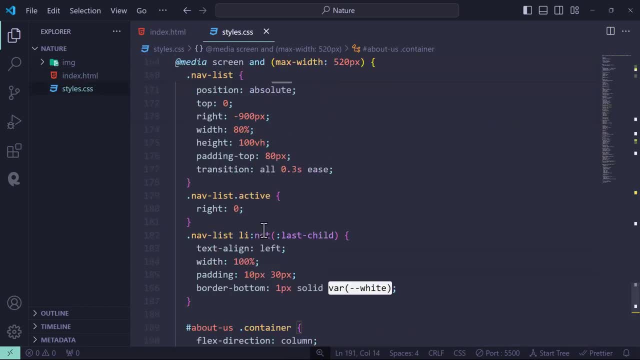 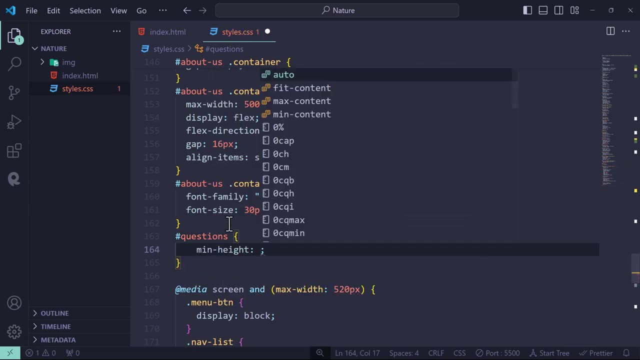 see, let's copy this ID at the top right here for the questions. let's add a min height of 500 pixel and for this we have a background image which is URL inside it. we have a background image which is URL inside it. we have a background image. 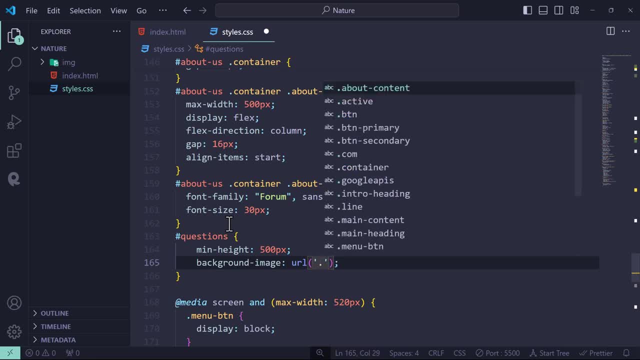 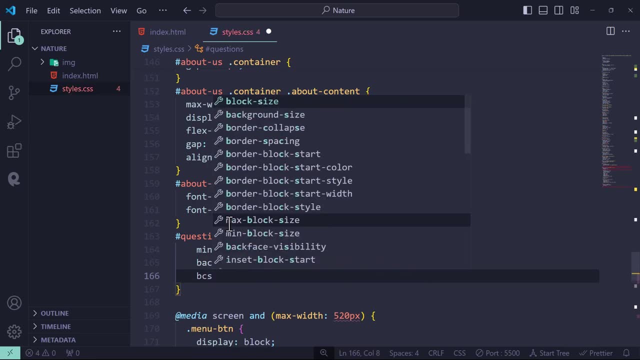 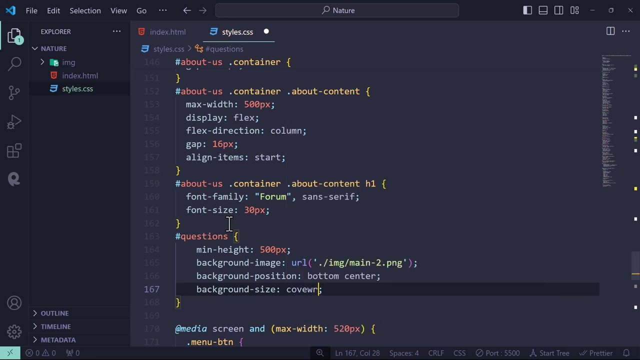 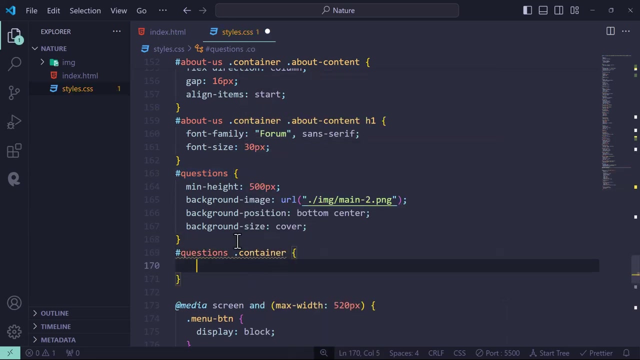 which is URL inside it. we have a background image which is URL inside position. position should be bottom center and background size. cover now. position should be bottom center and background size. cover now inside questions for the container. let's make max width to 500px and flex direction column and gap 16px and align items center. 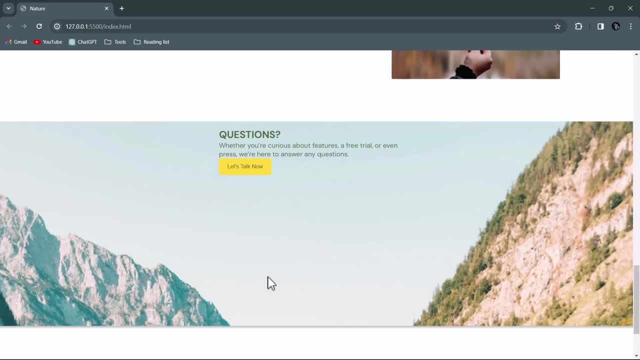 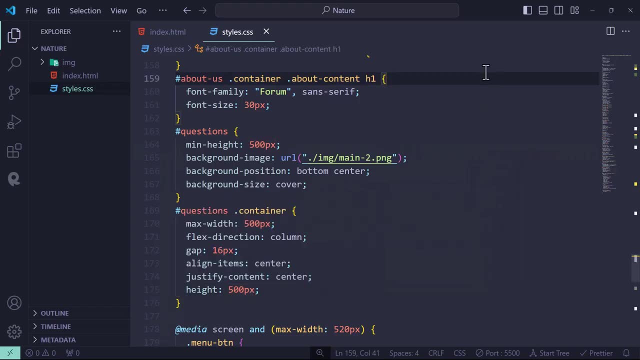 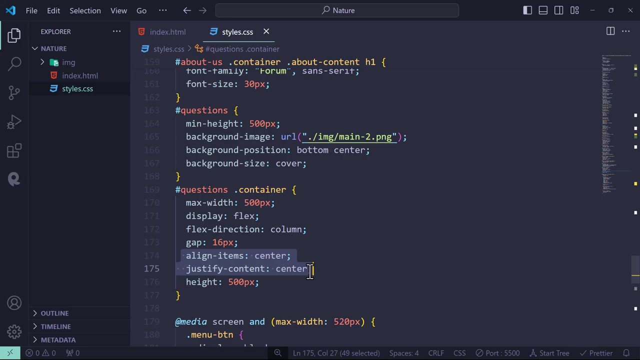 and justify content center and let's make height to 500px. we have to make display flex. only then flex direction, align items and justify content will work. you can see this was in center and inside this questions for the h1. let's make font size to 50px. you can see we 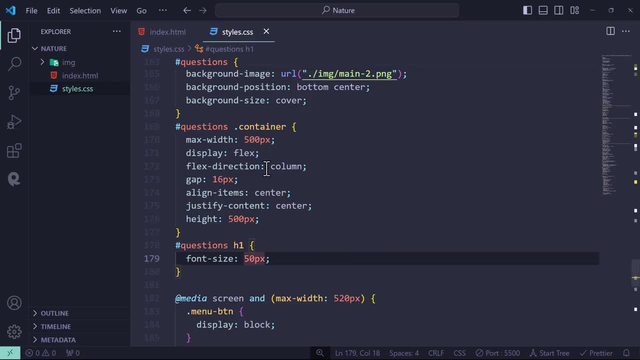 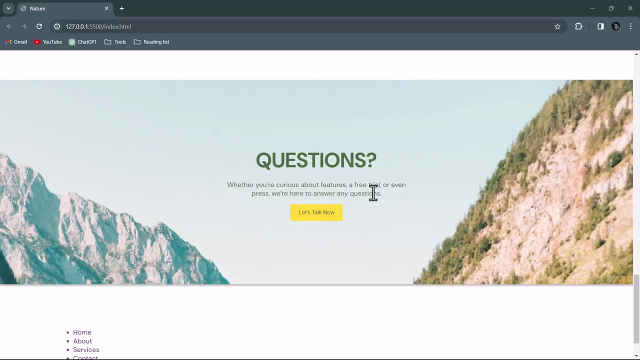 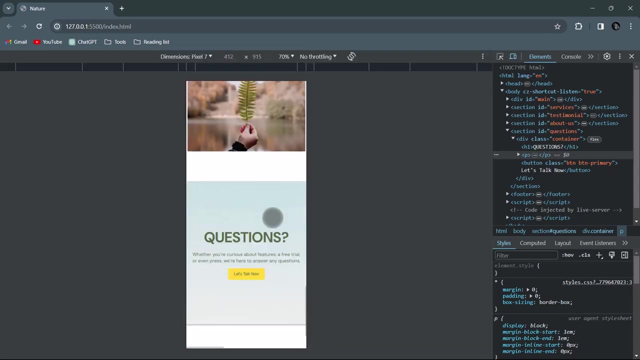 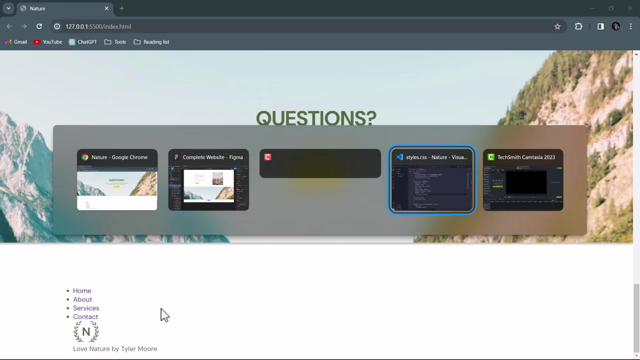 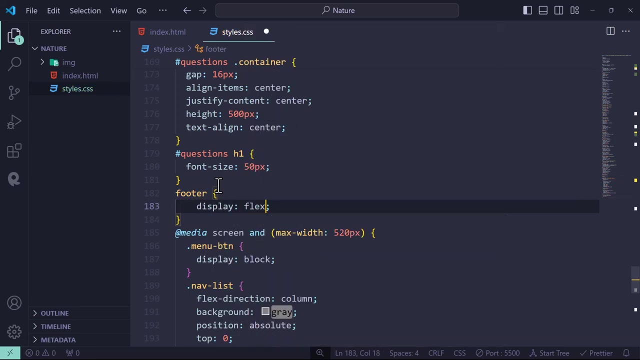 have this beautiful question section also and for this, make text align to 500px and to center. now let's open this inside mobile. now you can see how beautiful question section also. now let's style our footer. so for the footer, let's make display as flex and let's 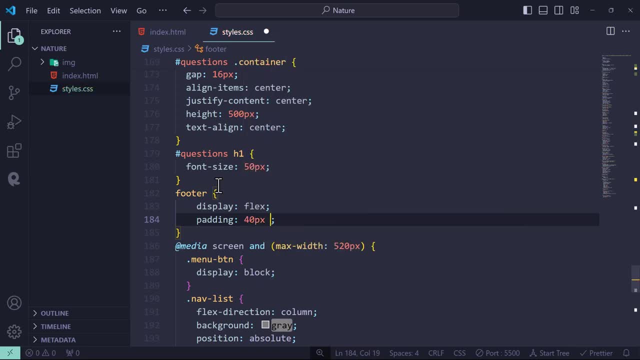 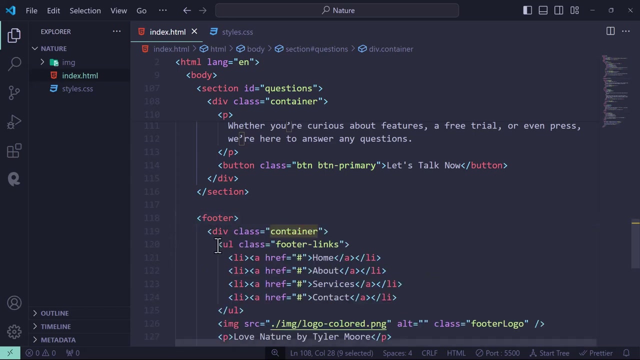 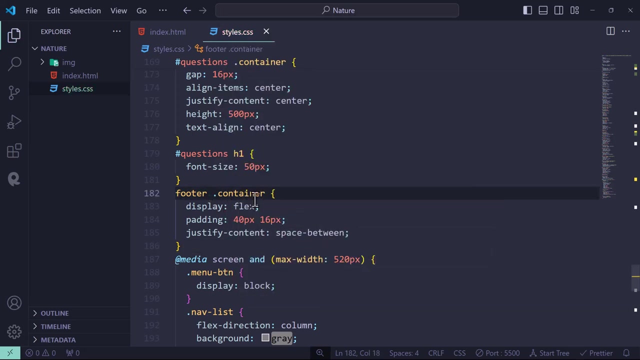 add some padding top and bottom. this means we have to make this font size to 40px and left and right 16px and justify content space between. as you can see, inside the footer you have this container, so i have to apply out of the styles to that container inside this footer for the container. as you 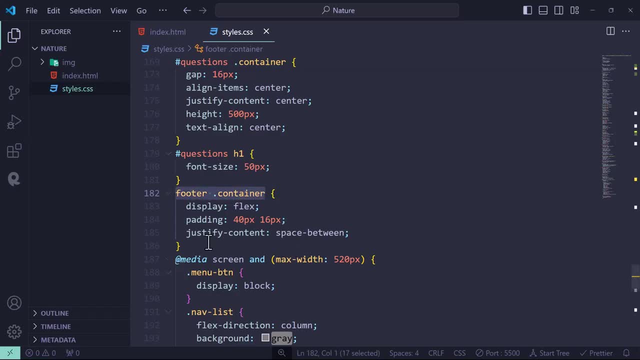 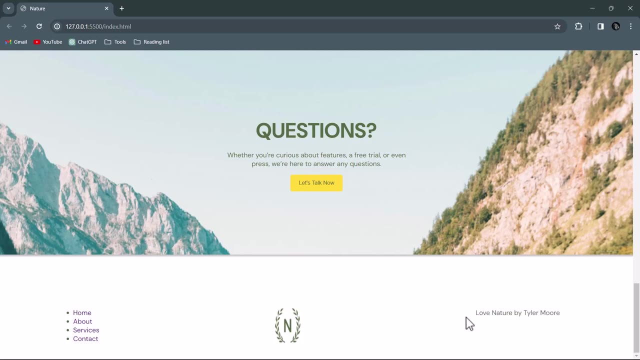 can see. as you can see, this one is six slab row. it's one small table and it's a bit narrow. it's nav links at here, logo in center and this footer text is at the end. so if you make align items center, so this will be aligned in center. so for the footer list, 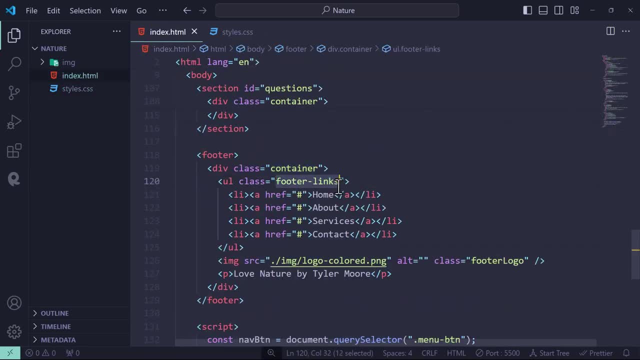 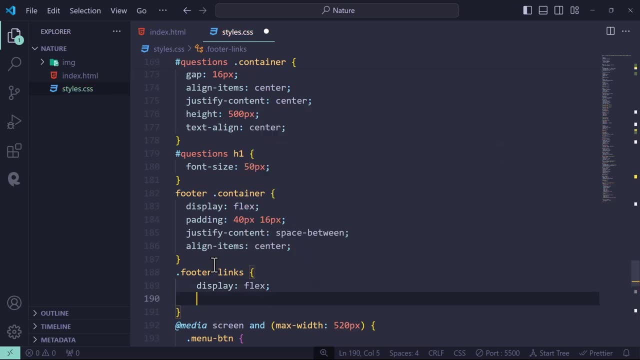 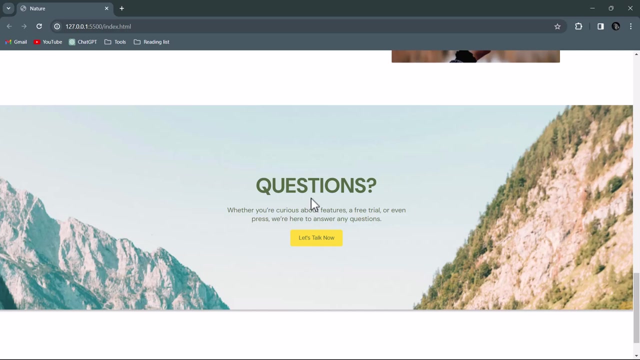 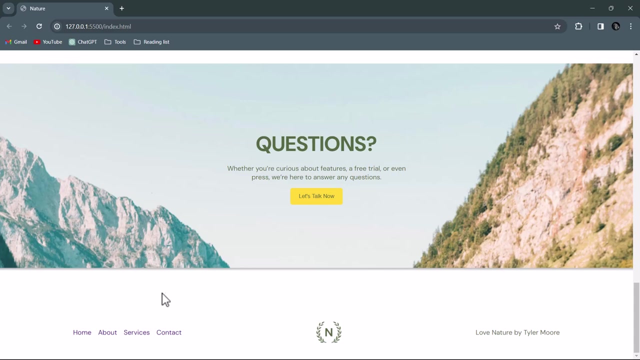 so inside this footer, footer links, if you make display as flex line, items center and a gap of 16 pixel and list style: none and, as you can see, our questions is a section by default. we added a margin top and bottom to all of our sections, so we have this extra 60 pixel, 60 pixel of margin margin bottom.